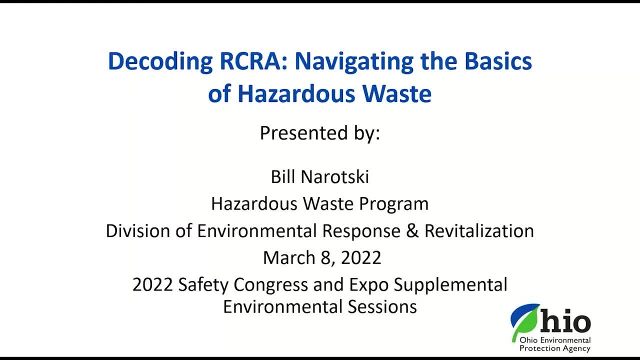 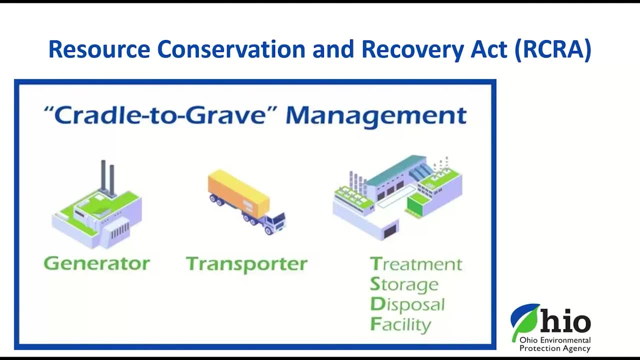 links to our webpages. They are in blue font and underlined, which making the notes a useful tool, And we recently updated our webpages, so the links may be really helpful. The Resource Conservation and Recovery Act, or RCRA, is what regulates hazardous waste. 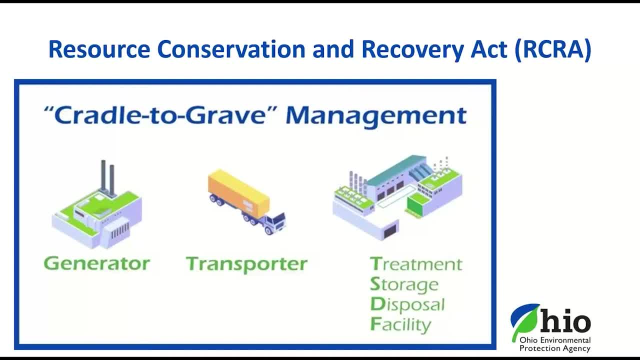 from the moment it's generated at a place of business until its final disposal, which is why we refer to it as cradle-to-grave management. Specifically, RCRA subtitle C is what regulates hazardous waste. There are rules for generators, but most businesses 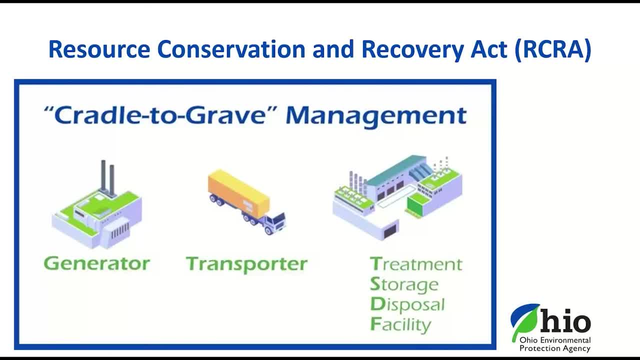 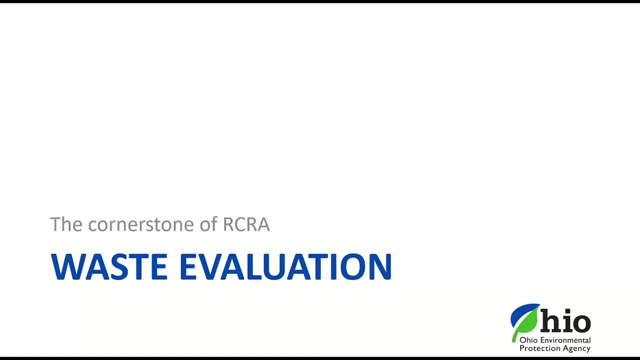 probably R transporters and permitted treatment, storage and disposal facilities. For this presentation, we are focusing on generator requirements. In order to understand if you are subject to RCRA, you really have to know if you are generating hazardous waste And 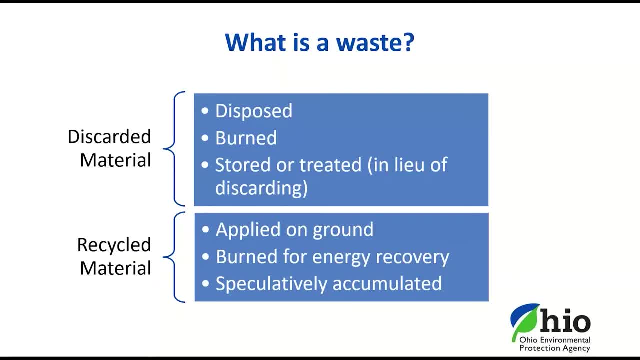 for a material to be a hazardous waste, it must first meet the definition of a waste. A waste is a material that will be discarded and used as a waste. A waste is a material that will be discarded and used as a waste. A waste is a material that will be discarded and used as a waste. A waste is a material that will be discarded. 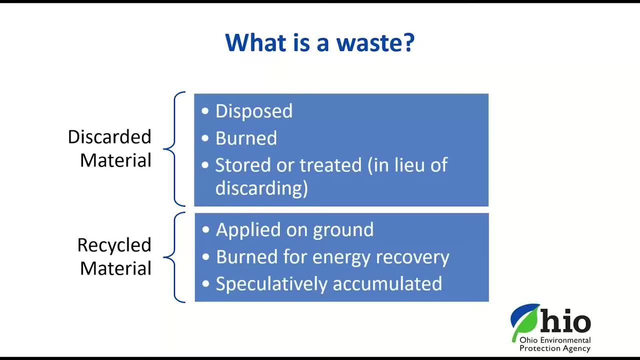 either by disposal, by burning, by storing or by treating that material in lieu of discarding it. A waste is also any material that will be recycled, either by using on or applying to the ground or burning it for energy recovery, or if it's speculatively accumulated for the intent to recycle. 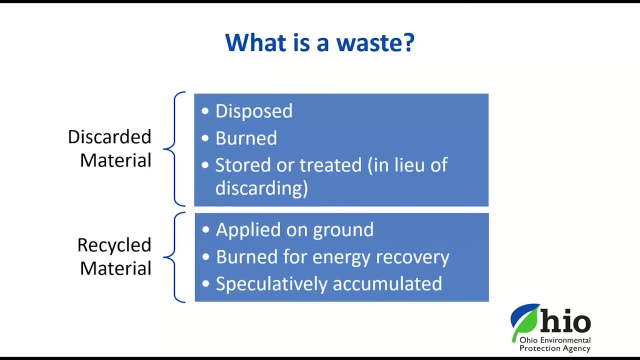 Speculative accumulation is demonstrated when a recycler does not recycle at least 75% of the material in a calendar year. The more that it is dug, the more a every concrete piece of a material will be discarded, dragged outами discarded during the cycle. 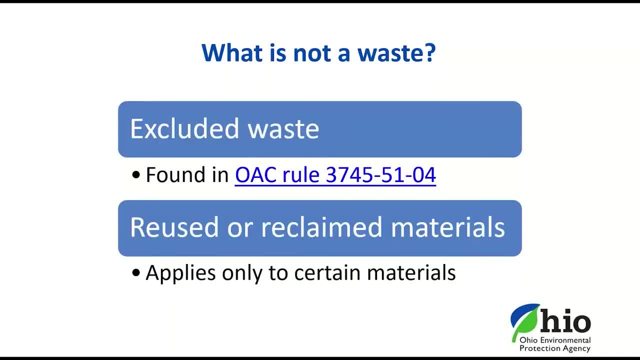 The more it is dug, the more a rechargeable material will be wagged off into the river. Certain things are not considered wastes. If they are specifically excluded by role, or when certain materials will be reused or reclaimed, they are not considered wastes. 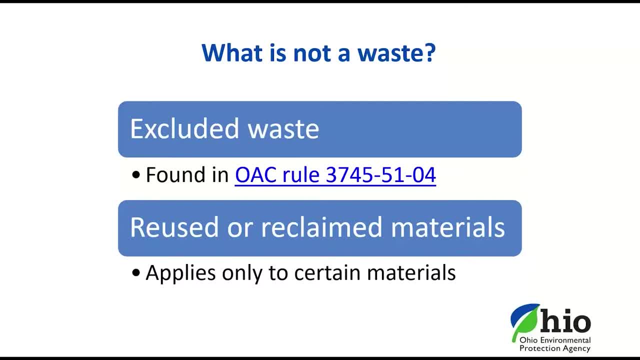 But keep in mind that many materials, including spent materials or listed byproducts, are wastes even when they are reclaimed. As I mentioned before, if a material is put on the land, the O 삼 bas unsamskiencehally nlawir V tiverpaz, Только naf tsa pi auspaar Está. keep in mind that when materials are used, they are waste only if they are reused or reclaimed. 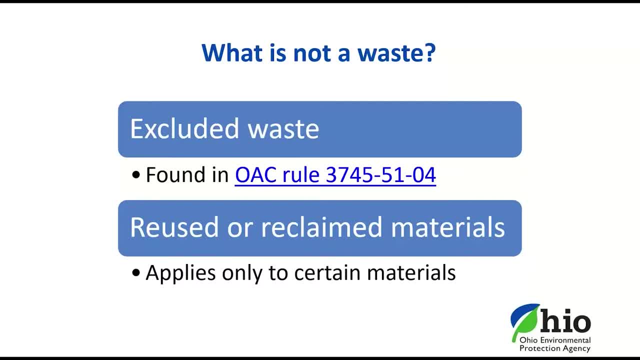 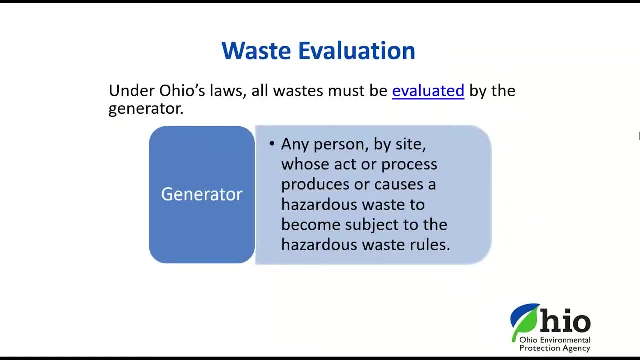 put on the land burned or speculatively accumulated, it is considered a waste. ohio's waste laws specify that generator is any person by site whose act or process produces a hazardous waste or causes a waste to be subject to the hazardous waste rules. and again, in order 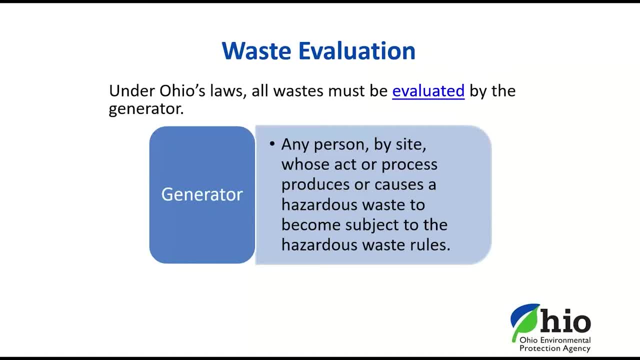 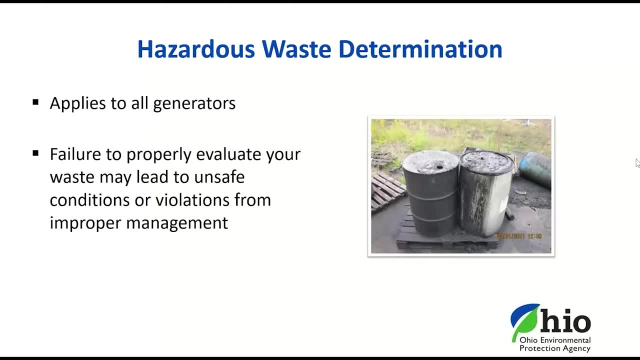 for a material to be a hazardous waste, it must first meet the definition of a waste, and if you generate a waste, you must determine if your waste is a hazardous waste. ohio administrative code or oac roll. 3745 5211 provides you with the step-by-step procedures to make. 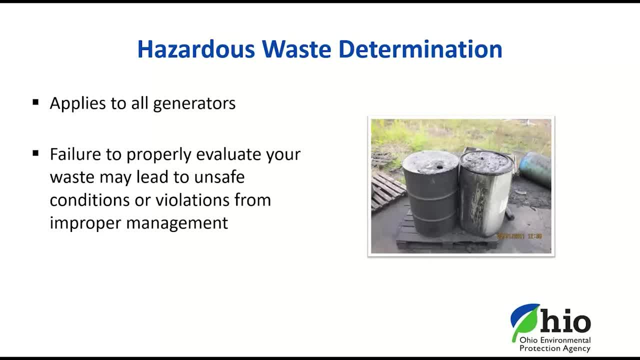 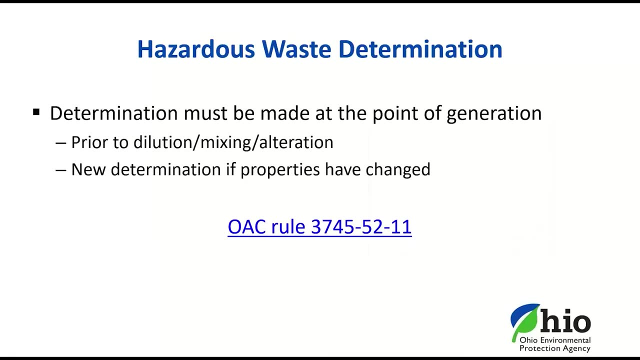 when to follow when making this determination. failure to properly evaluate your waste may lead to unsafe management, treatment or disposal of hazardous waste, so proper waste evaluation is very important. a waste determination needs to be made at the point of generation, prior to any dilution, mixing or alteration, because those activities could change the properties of the waste. 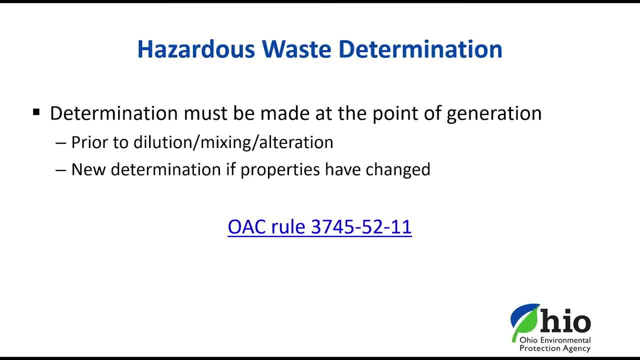 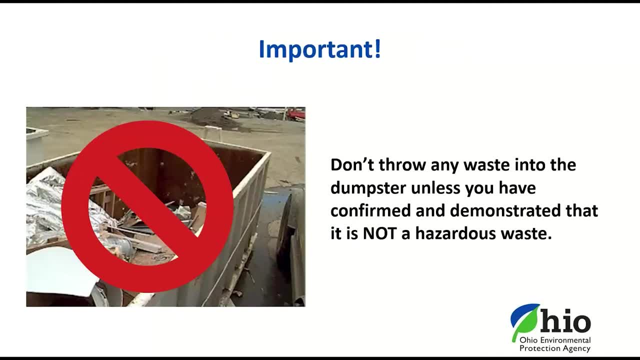 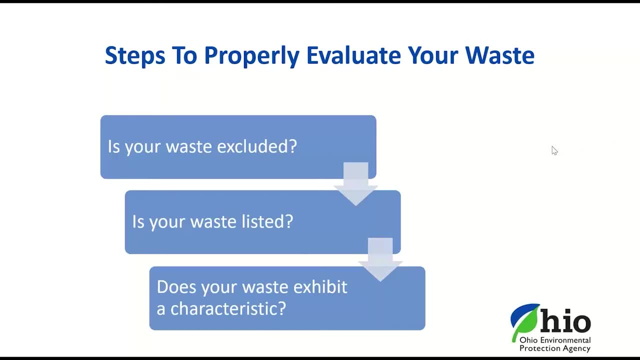 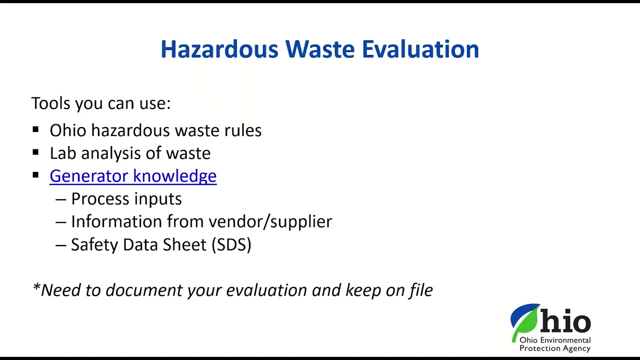 anytime the properties have changed, a new determination needs to be made. so don't throw any waste into the dumpster until you've determined that the waste is not hazardous. some options that are available to make waste determinations include the hazardous waste rolls. thanks to the roles are on the downloadable presentation notes. 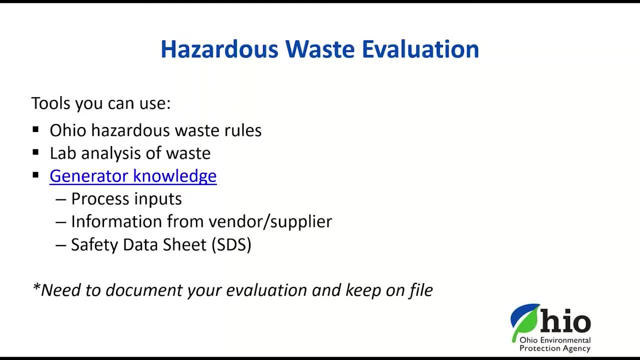 you can collect a representative sample of your waste and submit it for analysis at a lab, or you can use your knowledge as a generator. the rule doesn't specify what sources you can use as generator knowledge, nor does use epa have any formal guidance. but some of the things you 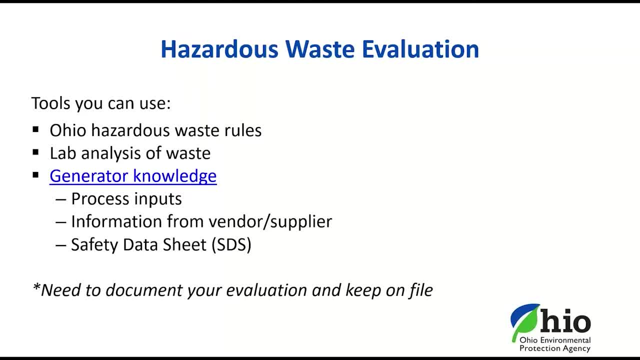 can consider are your process inputs, the raw materials. you are using information provided by your supplier, and you can also reference safety data sheets. however, you should be careful in using safety data sheets and you should be careful when using safety data sheets. and you should be careful when using safety data sheets. and you should be careful when using safety data sheets and you should 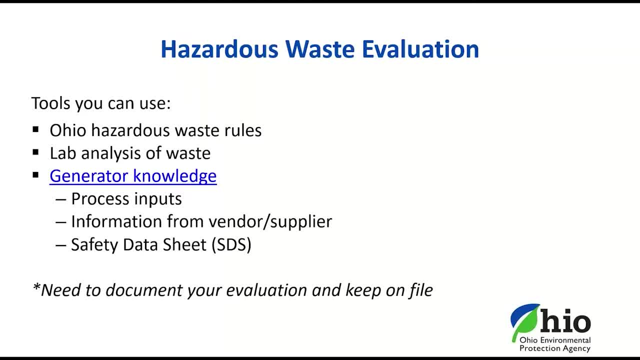 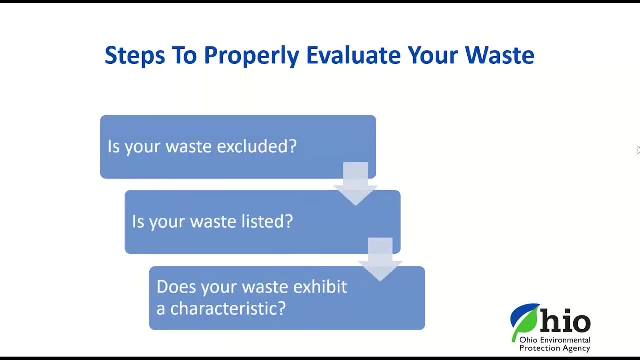 never be used as the sole determination, but more used more as a supportive document, because they don't always list all hazardous constituent levels and some things may be a trade secret. the basic questions you need to ask when making a waste determination are: is this waste excluded? does it belong to a specific waste list? 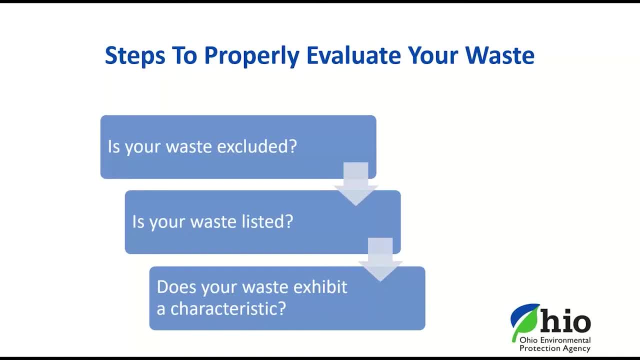 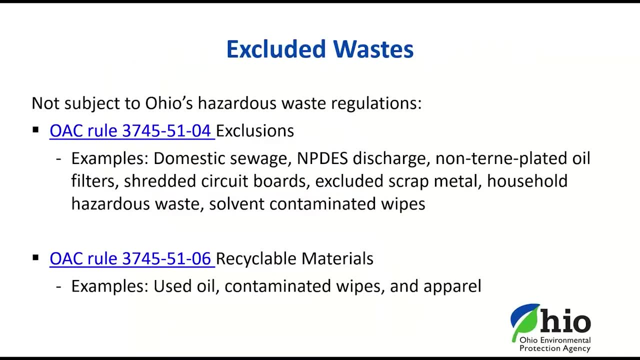 and i'll get to the fkp and you list in a moment- and does the waste exhibit a hazardous characteristic? the first thing you want to do is look at oac roll 3745 5104. this rule lists and describes the specific wastes that are excluded from hazardous waste regulation. 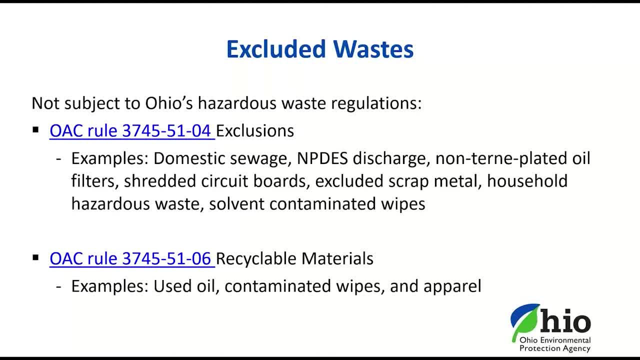 as well as any conditions they need to meet. there are about 34 pages of exclusions, and some common examples are provided on the slide. you then should also look at oec roll 3745 5106, which defines additional exclusions and requirements for recyclable materials. 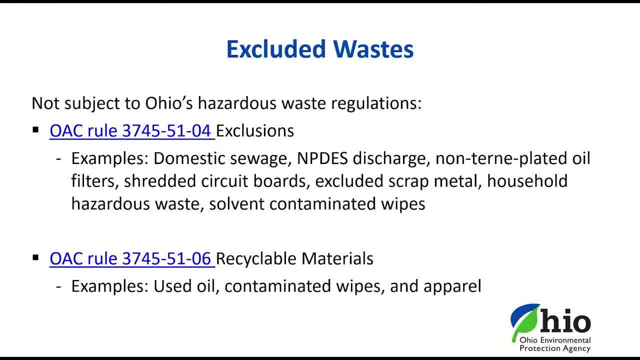 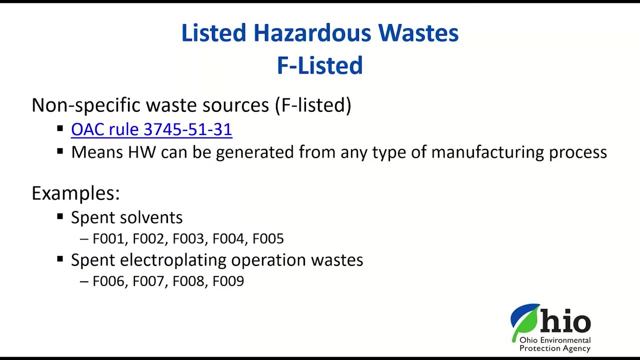 including used oil and contaminated wipes and apparel- also referred to as hazardous textiles- that will be laundered and returned to use if your waste does not meet an exclusion. you want to take a look at the four hazardous waste lists. the first one we are going to talk about is the f list. these hazardous weights come from. 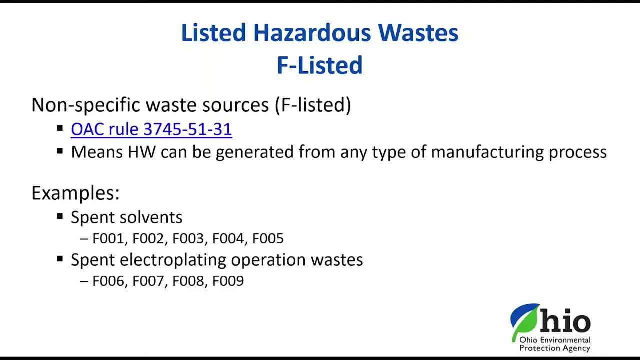 non-specific sources, which just means that they can be generated from a wide range of manufacturing processes. some in common examples are spent solvents such as trichloroethylene, xylene and toluene, as well as electroplating wastes such as waste water treatment sludges and plating bath solutions or residues. 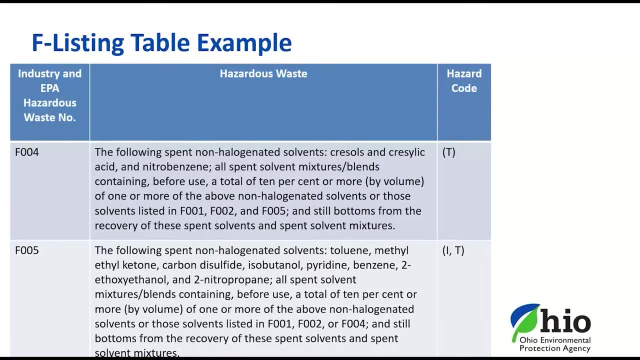 here is a snapshot of part of the f list table. you can see the waste number is in the left hand column and in the middle there is a description of the waste that falls into that category, and the right hand column has a hazard code which indicates the reason for listing the waste. 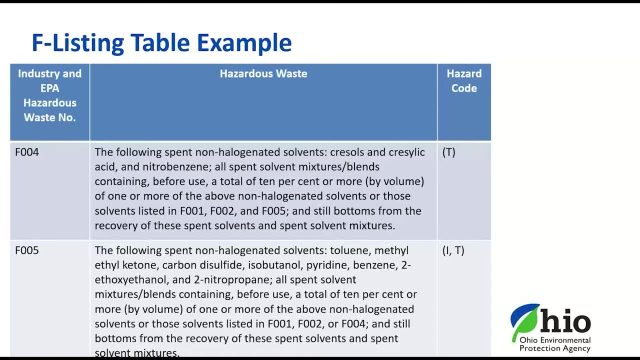 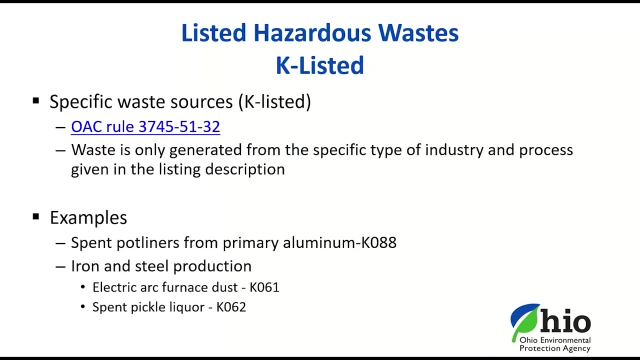 there are several hazard codes that you may see listed, including t for toxic waste, h for acute hazardous waste, i for ignitable waste, c for corrosive waste, r for reactive waste and e for toxicity characteristic waste. so we'll start with the a list. the next list is the k list, which is industry specific. some examples include spent pot liners. 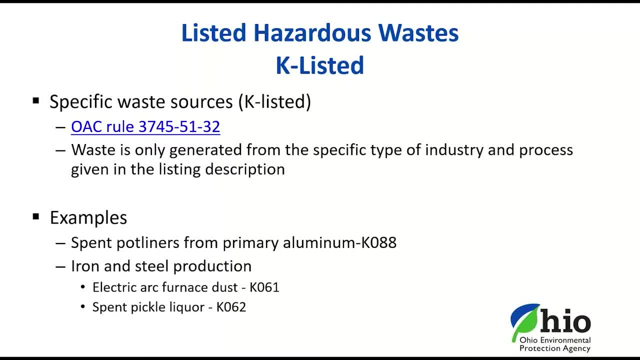 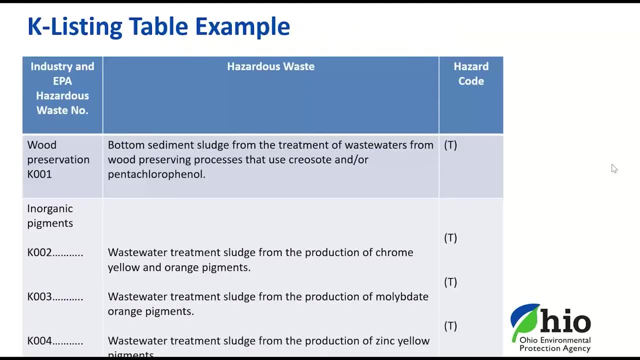 from primary aluminum reduction, as well as emission control dusts or sludge from steel production. this table shows some of the cases of these models listed wastes, as you can see in the hazardous waste description column there are. they are very source and industry specific. once again, the right column is letting you know why that waste belongs. 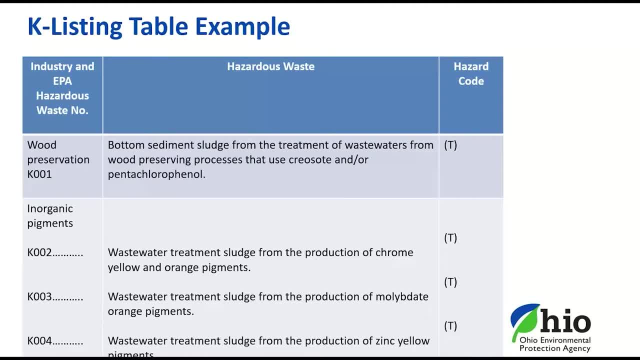 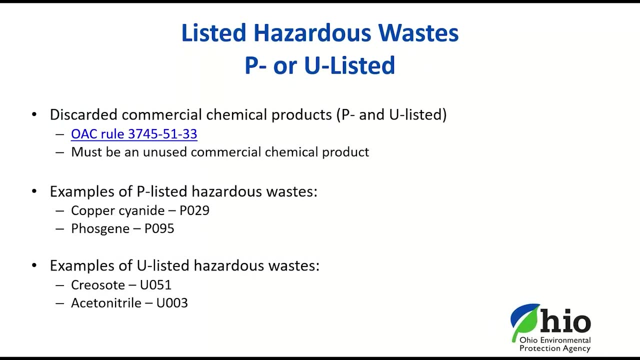 to this list and in the case of the ones provided on this list, they are all coded t, indicating toxic waste. the final two lists are the p and u lists, which contain unused discarded commercial chemical products. the key word here is they are unused, so if a waste was generated after going. 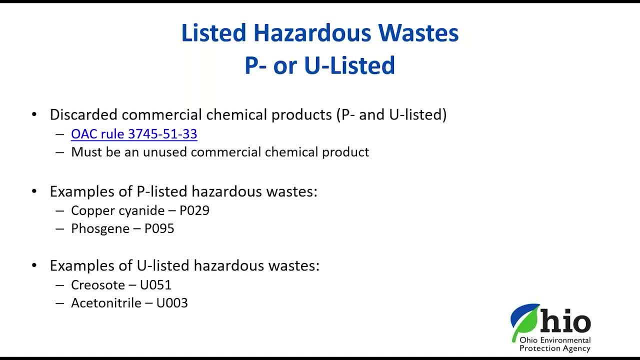 through a manufacturing process, it's not going to meet that requirement. the only difference between the p and u lists is the p list identifier of the decorum definition of waste. the p and u lists are used to identify hazardous waste and later also include um down and plus the p and u lists which include dangerous waste. 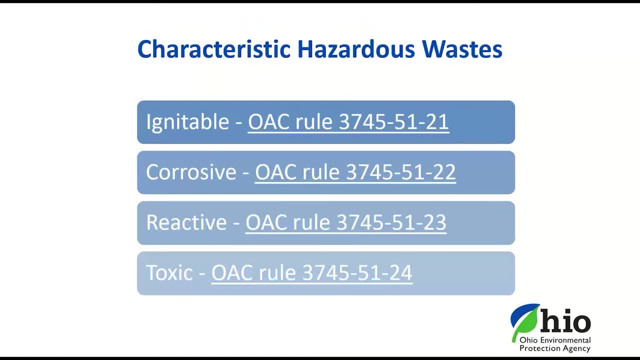 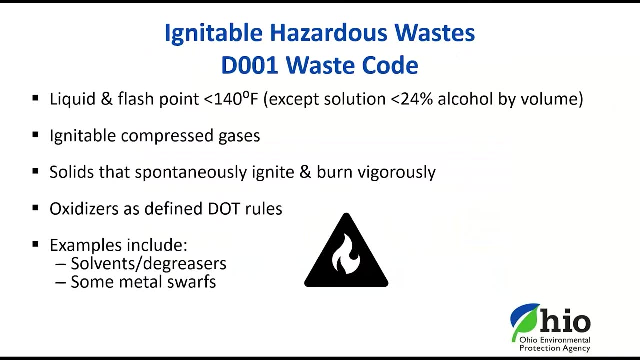 and well. we are using the p and u lists to identify acute hazardous wastes which are more dangerous in smaller quantities. now we are going to talk about the final step in making a hazardous waste determination. a waste can be hazardous if it exhibits a characteristic by being ignitable. 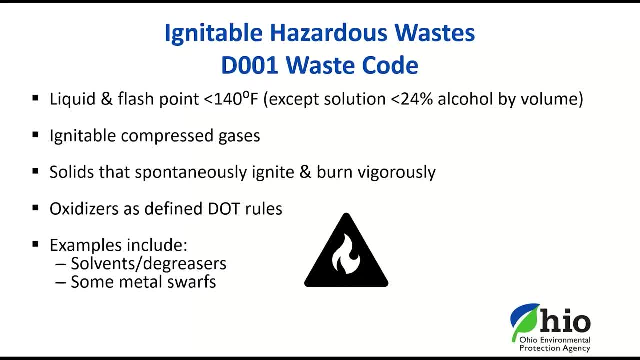 corrosive, reactive or toxic ignitable wastes are assigned the d001 and d002gor 3 and 5 for the carbon recompILES HOWS, IT, WILL, TECHNOLOGY, THE RECON framework ó on the site wwwucdedugovus waste code. These are liquids with a flashpoint of less than 140 degrees which include solvents. 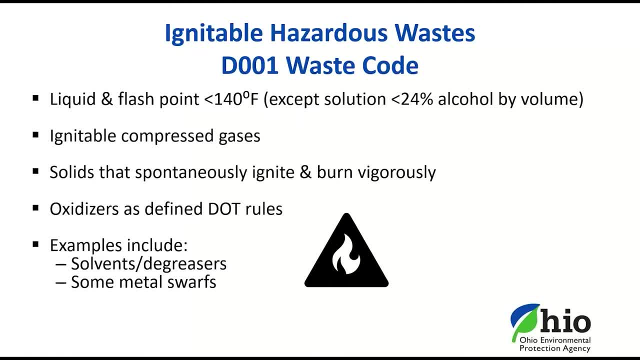 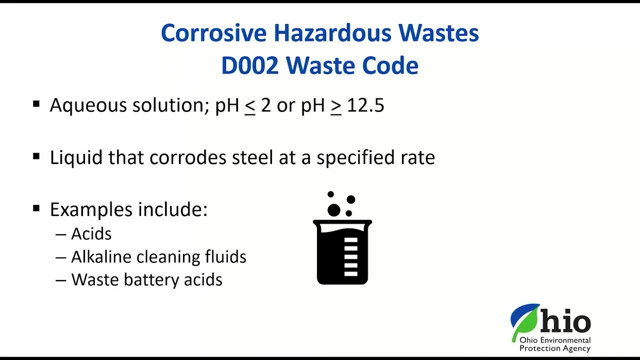 and degreasers. solids that spontaneously ignite, such as some metal swarfs and ignitable compressed gases and oxidizers. Corrosive hazardous wastes carry the D002 waste code. These are acids and acids Alkyl solutions with a pH of less than or equal to 2 or greater than or equal to 12.5.. 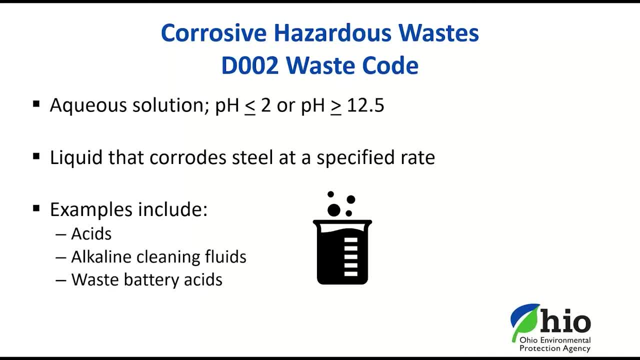 These are liquids that corrode steel at a specified rate. So you really want to know if your waste is corrosive, because it's going to determine what type of container you can use to store it. Some examples include sodium hydroxide and waste hydrochloric acid. 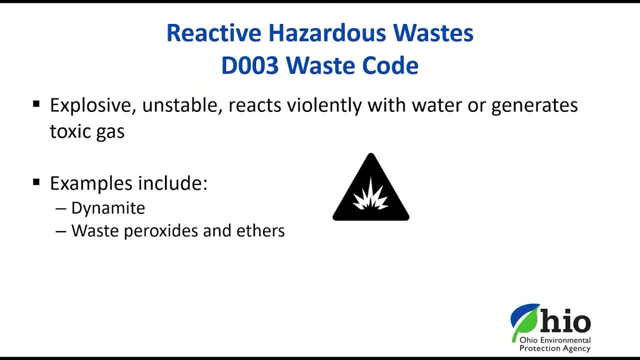 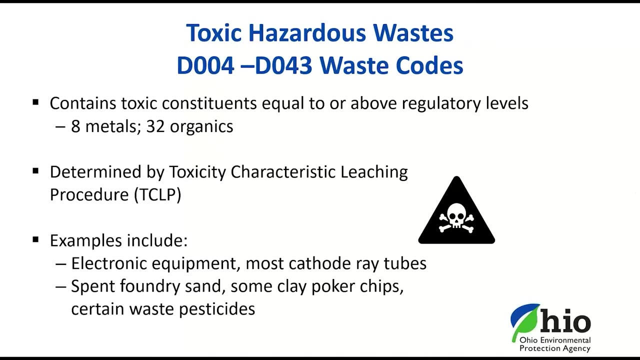 Reactive hazardous wastes will carry the D003 waste code and they are extremely unstable. These wastes can explode or react violently with water. An example is ammonium nitrate. The fourth category of characteristic hazardous waste is for toxicity, While the previous three categories have the potential to cause an increase in toxicity, the next category of waste is for 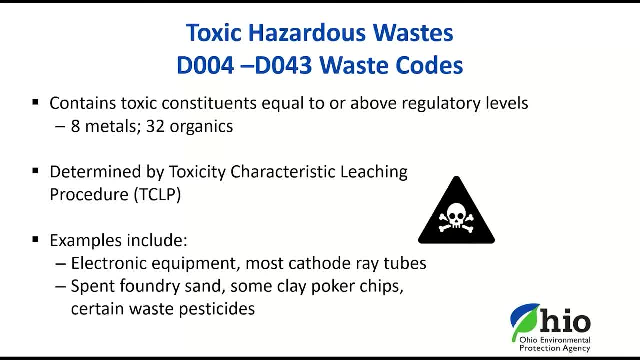 toxicity. The fourth category of characteristics of hazardous waste is for toxicity. while the previous three categories have the potential to cause an increase, in toxicity cause more of an immediate harm. Waste that are characteristically toxic also have the potential to cause long-term harm by contaminating our groundwater. The waste code ranges from D004 to. 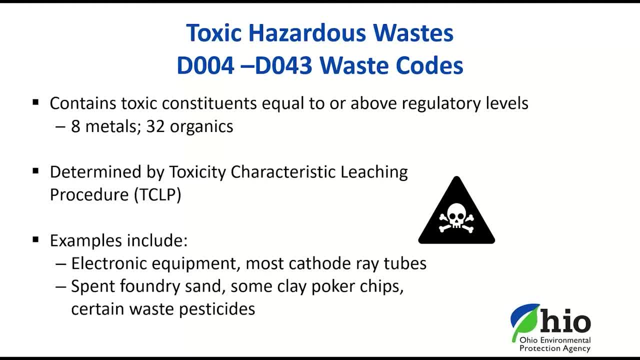 D043.. To determine if your waste is toxic, take a representative sample of the waste and send it to a lab for toxicity characteristic leaching procedure or T-clip analysis. The lab will simulate landfill conditions to determine the amount of chemicals that will leach into the. 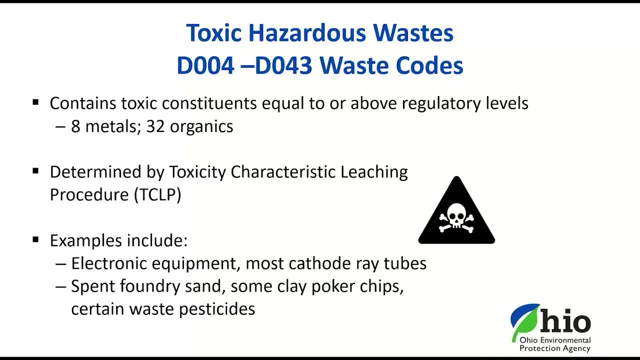 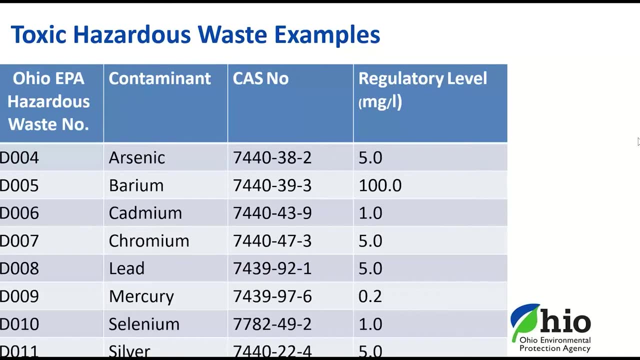 groundwater. If the waste contains toxic constituents equal to two or greater than the regulatory levels, you have a waste characteristic of toxicity. There are 32 organics in this category, as well as eight recrimetals. This table shows the waste codes. 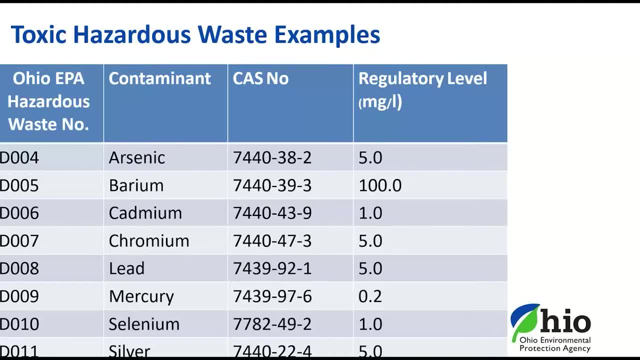 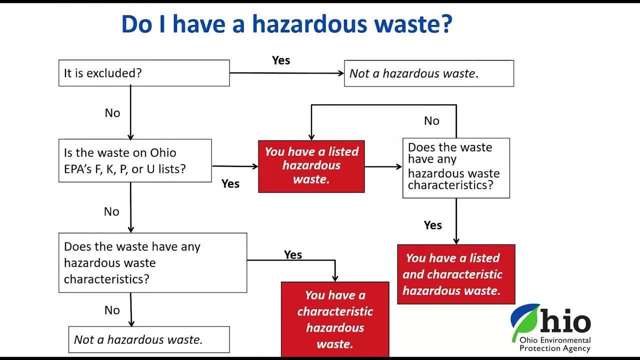 on the left and the regulatory levels in milligrams per liter on the right. Once you get your lab results back, you can compare the results to this table to determine if you have a hazardous waste. So let's take a moment to recap the waste determination process. 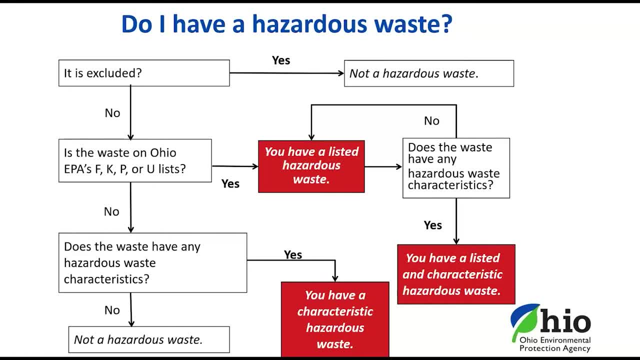 First, is it excluded? If it is, then you don't have a hazardous waste. If not, you need to move on to examining the four hazardous waste lists, As you can see by this chart. even if you determine that you have a listed hazardous waste, you cannot stop there. You still must. 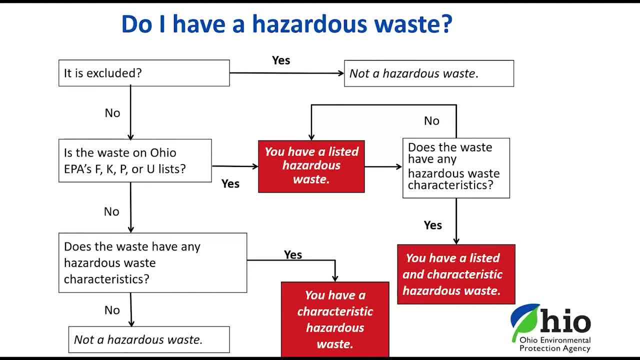 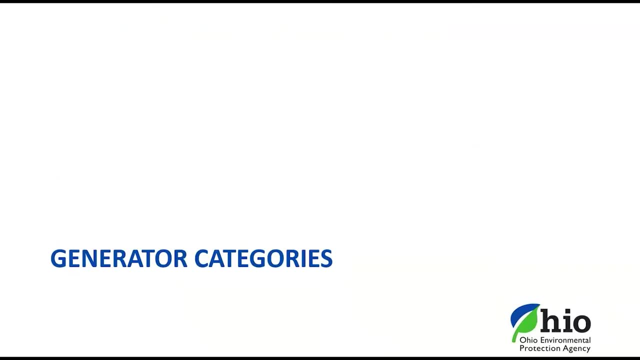 determine if the waste also exhibits a characteristic. If the waste is not listed or characteristic, you're done. Just keep the determination on file. Once you've determined you have a hazardous waste, you have to know the size of the generator you are, because that's going to determine. 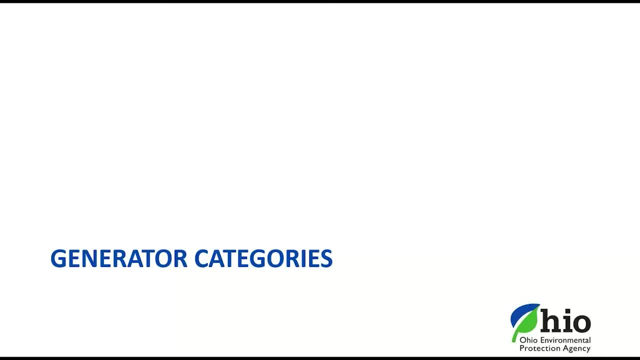 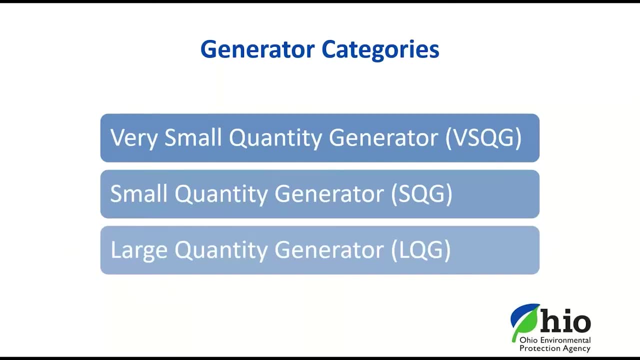 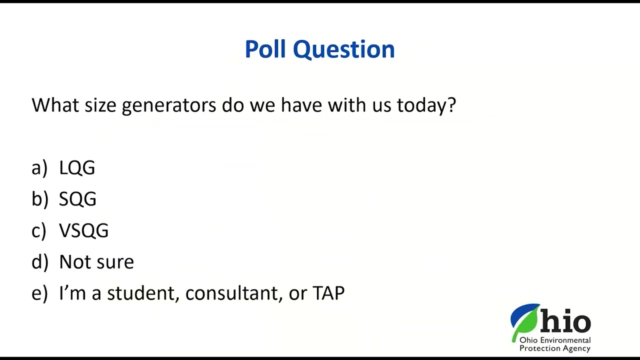 what type of requirements you need to follow. For Ohio and most states, there are three different generator categories that are based on how much you generate in one calendar month, as well as how much you store on site. So let's get to our first poll question and see. 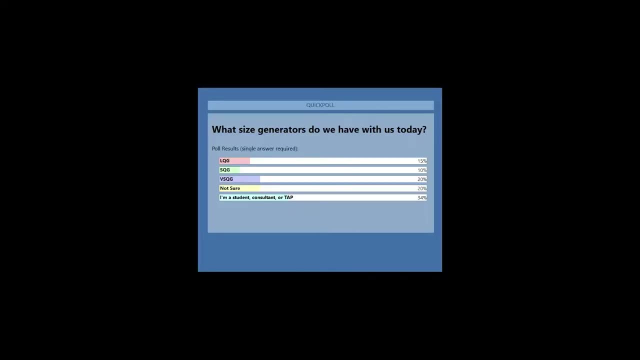 what size generators we have with us today. Thanks, Helen. Looks like we have a pretty good mix and there's quite a few consultants and TAPs for students on, so hopefully the presentation will be good information for you and a useful toolkit for you this year. Thanks, 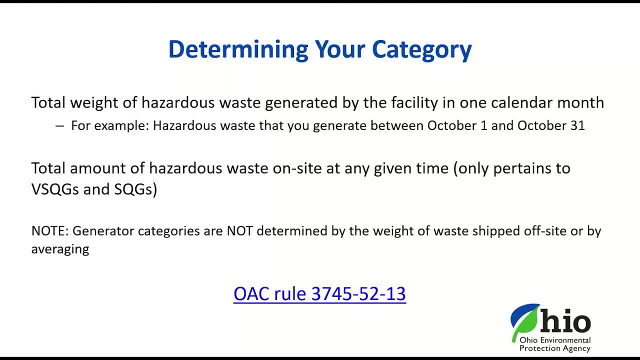 When determining your generator category, you must count the total weight of all hazardous waste generated at a facility in a calendar month. Very small quantity generated and small quantity generated or smaller generators. and smaller quantity generators are also limited in how much hazardous waste they can store on site, So you will want to pay. 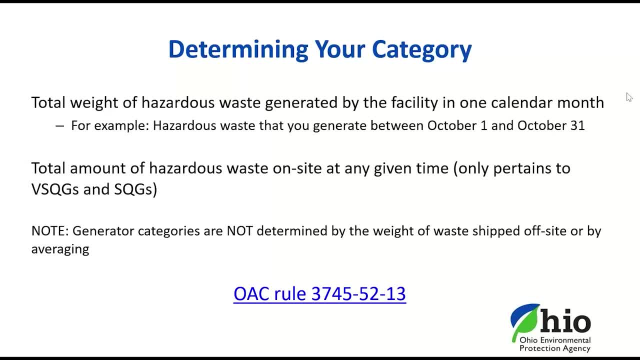 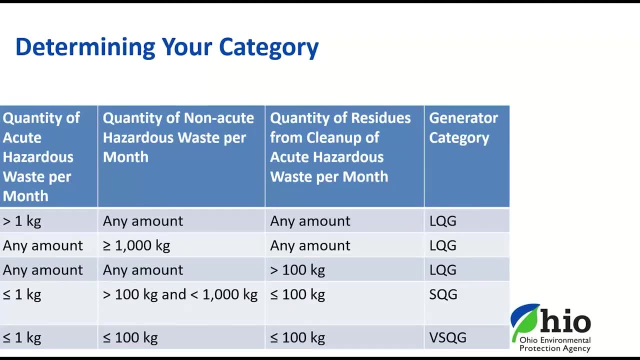 attention to those numbers as well. When a generator is determining their generator category, they must consider three relevant types of hazardous waste: Hazardous waste or non-acute. hazardous waste for purposes of this discussion. Acute hazardous waste or non-acute. 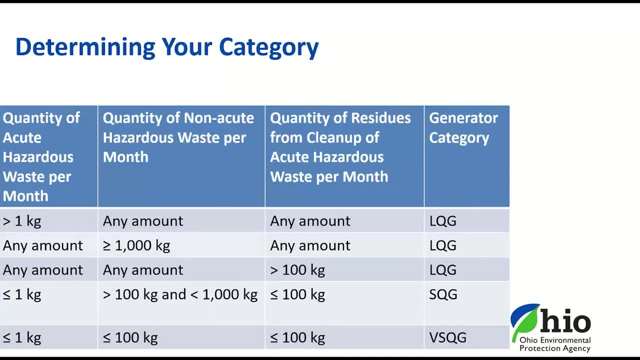 improved hazardous waste for purposes of this discussion And as always, please note no waste and residues from the cleanup of a spill of acute hazardous waste. in three of these, in three of the scenarios here on the slide, the generator is a large quantity. 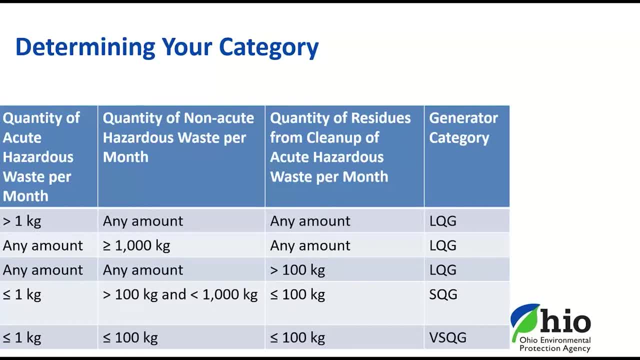 generator. in one scenario, the generator is a small quantity generator and in one, a very small quantity generator. when calculating generator categories, the quantities of acute hazardous waste and non-acute hazardous wastes are considered separately. you will want to pay attention to the limit for acute hazardous waste, because it only takes one. 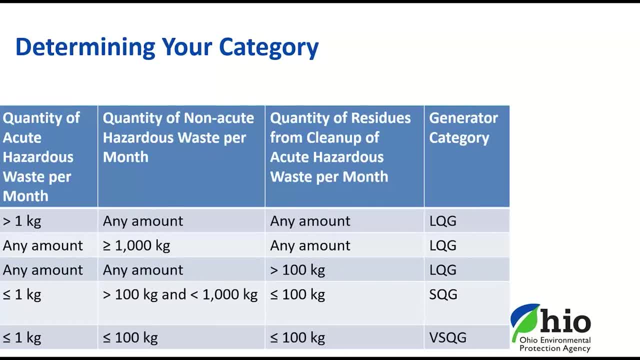 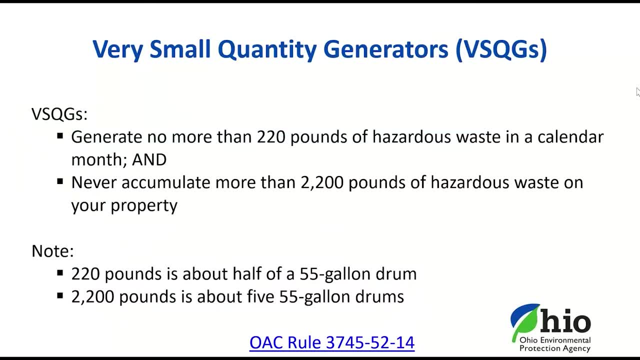 kilogram or 2.2 pounds of acute hazardous waste to make you a large quantity generator. very small quantity generators generate up to 220 pounds of hazardous waste in a month, which is roughly half of a 55 gallon drum, and never store more than 2200 pounds of hazardous waste. on site, which is roughly 5- 55 gallon drums. that, of course, is going to vary based on the density of your waste streams. the next category is small quantity generators. you will fall into this category if you generate more than 220 pounds but less than 2 200 pounds of hazardous waste in a calendar month. 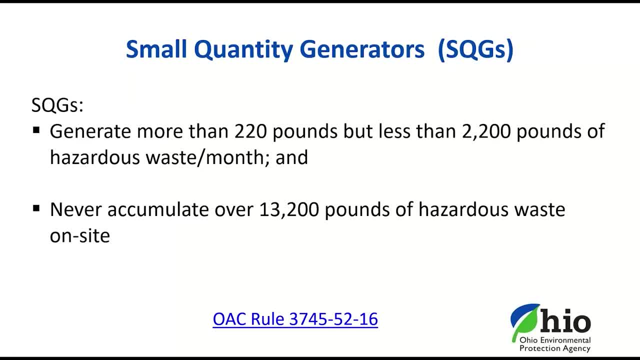 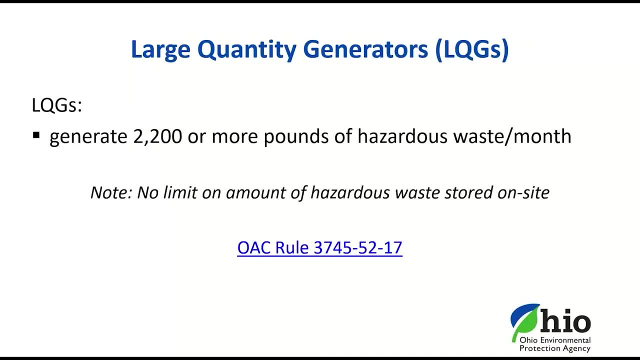 you are also limited to the amount of hazardous waste stored on site at any given time to 13 200 large quantity generators generate 2 200 pounds or more of hazardous waste per month and have no limit for generator status on the amount of hazardous waste stored on site. 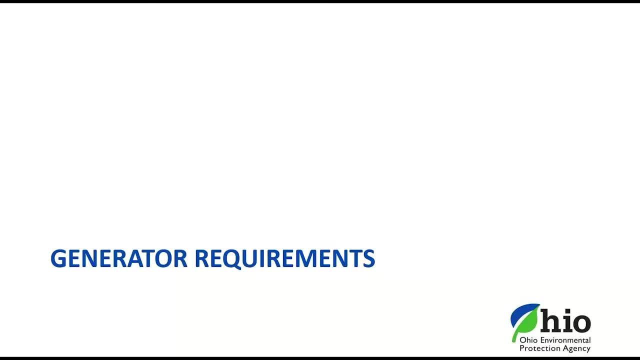 now we are going to get into the specific requirements that generators need to follow. i would like to re-emphasize that RCRA subtitle c was established to regulate the management of hazardous waste, which includes permitting. when we talk about all the specific requirements for the generator, 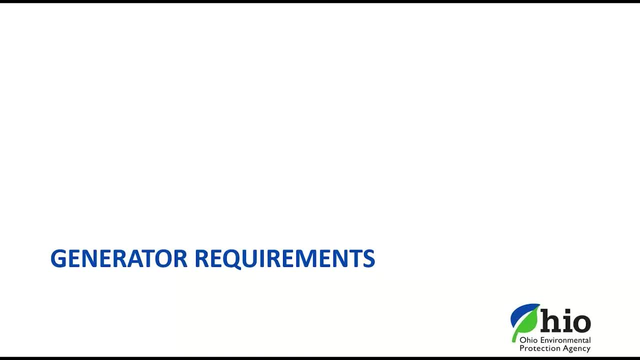 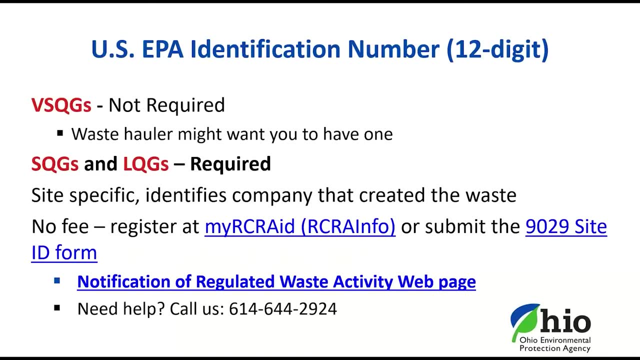 categories. these are conditions that must be followed in order to be exempt from permitting requirements, which are much more burdensome if you generate, treat, store or dispose of hazardous waste. recommend the focus on rep replies have a shadow of a turd who is givenzt that figure fairly 없어. category, a term that is, outused, the term to מד or carried on this using a standard term, grown from states for permanent to permanent space. it figures up for about one percentage of hazardous waste, resulting in an additional water standard that may fall off or periods of air established levels under the methods of cycle may increase if the cluster travels in several hundred tons, if not more. a sucker layer�i and so on. 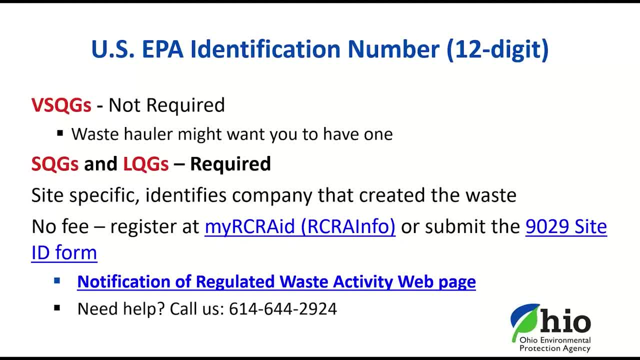 waste or store recyclable materials prior to recycling them. you may be required to notify Ohio EPA of your hazardous waste activity and obtain a US EPA identification number. you obtain this number by registering online through my rooker ID and recruit info, or by submitting form 9029 to Ohio. 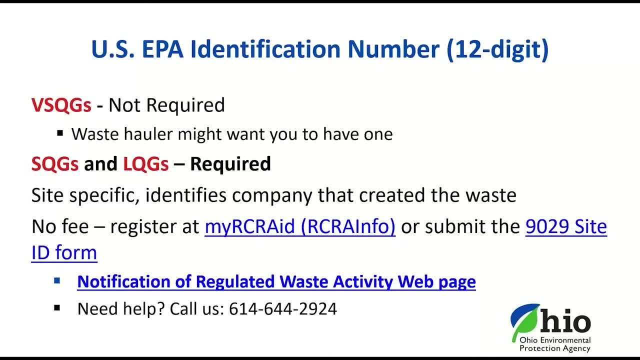 EPA. if you are a very small quantity generator, you are not required to obtain an ID number. but small quantity generators and large quantity generators need ID numbers. keep in mind ID numbers are site-specific, so you need to complete a form for each individual site that is required to obtain a number if your 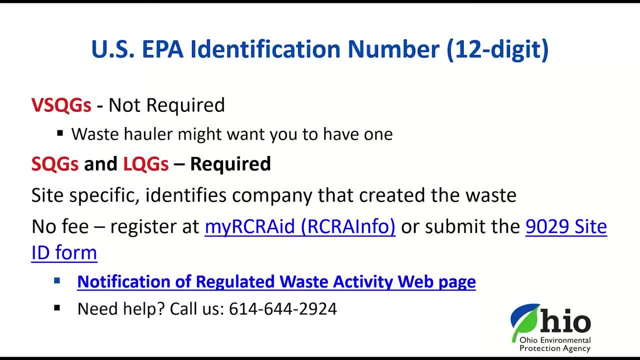 company moves to another location and will still be required to have an ID number. you must notify Ohio EPA of your new location and submit a new form. this is because ID numbers are not required to obtain an ID number. we also request that you submit a letter to deactivate the number at the 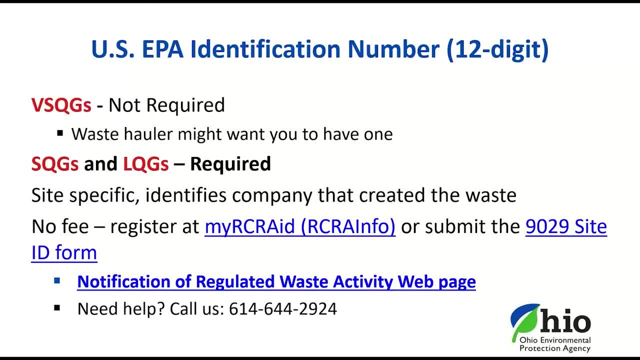 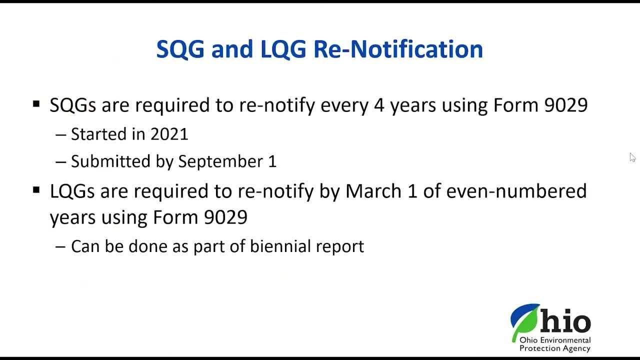 old site. it will be reassigned to future occupants if they generate hazardous waste. there is also a re notification requirement. small coin generators need to re notify every four years, submitting form 9029 by September 1st, again every four years. large quantity generators need to re notify March 1st of even years, which is 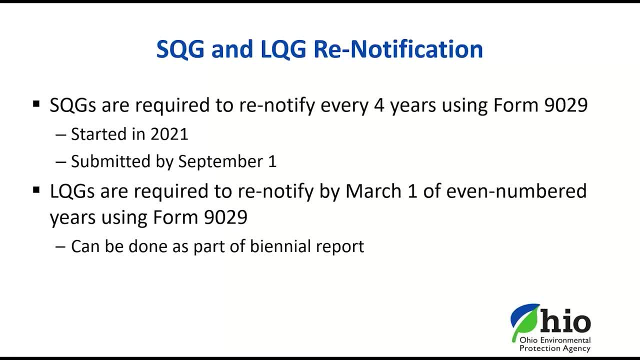 the same time biannual reports are due, so it can just be done as part of that report. since the deadline has just passed, I hope all the large quantity generators have re notified and if you haven't, please complete the renotification as soon as you can you. 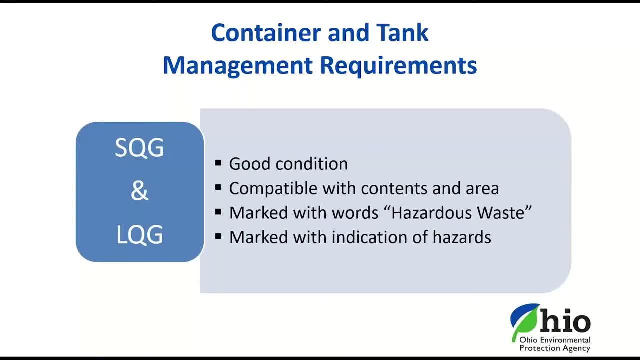 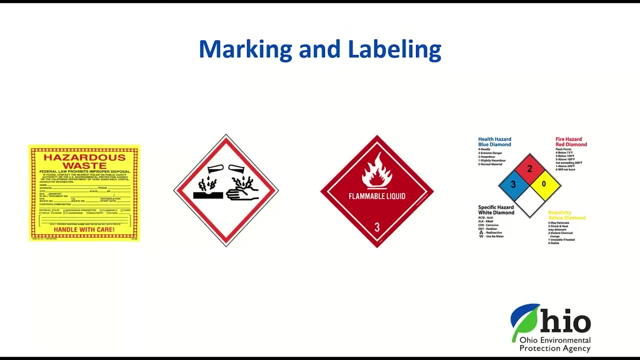 you. I will be accepting any questions that you may have in the Q&A box and I will be happy to answer any questions that you may have in the Q&A box. if you have any questions, please email me at the address on the slide. thank you, I appreciate the opportunity to talk to you today and I hope you have a great 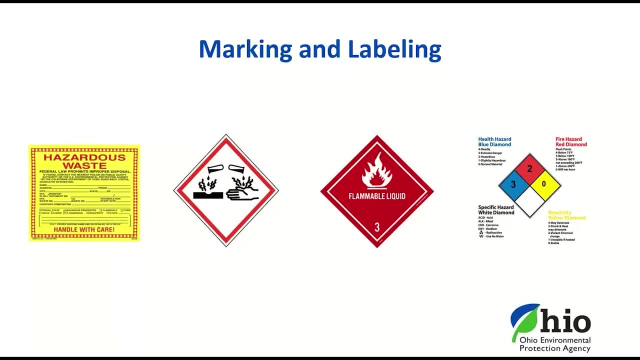 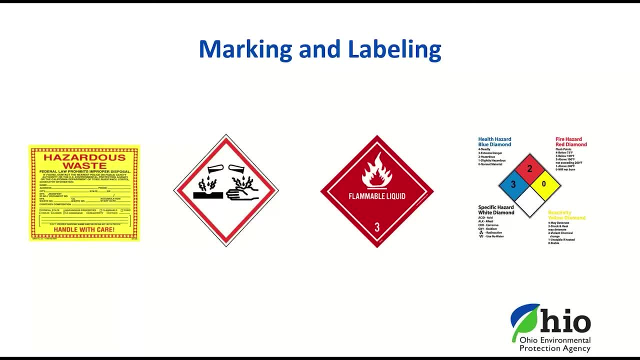 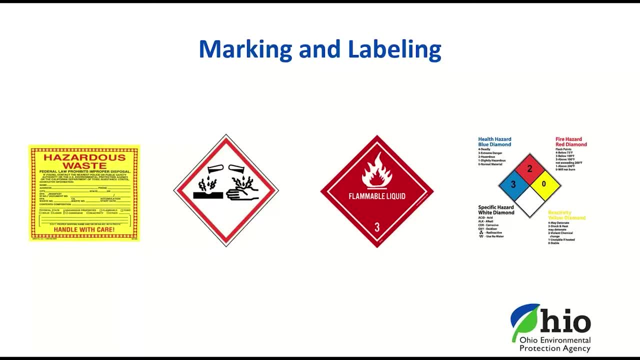 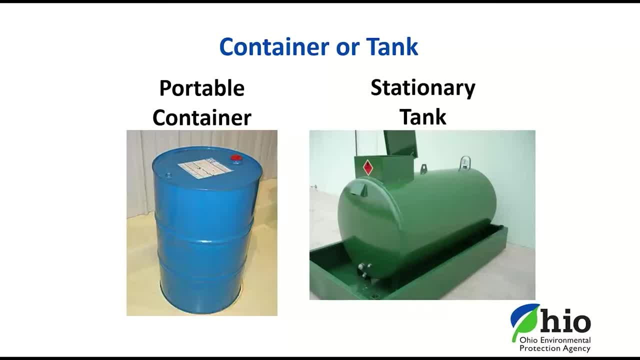 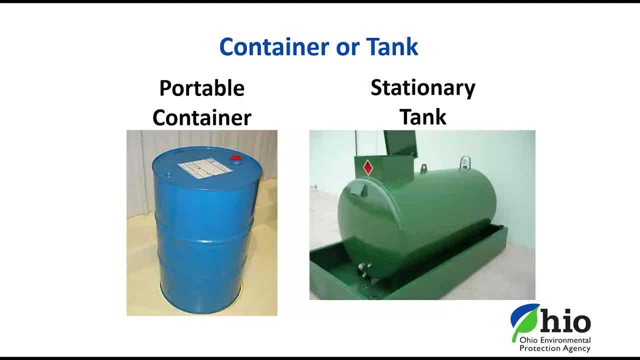 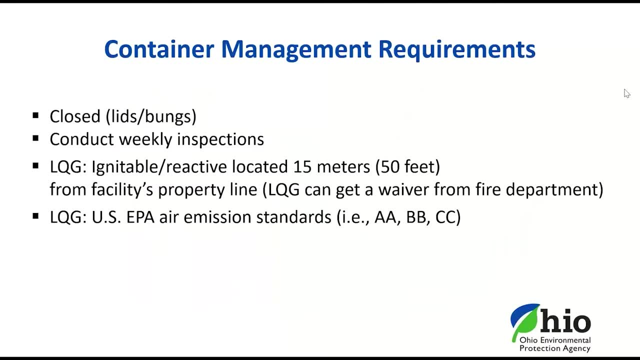 bye-bye, bye-bye. then moved to another location. it's a container. there are additional requirements for containers. lids need to be kept closed except when adding or removing waste, or venting if necessary, and containers need to be inspected weekly. if you are a large quantity generator, you also need to. 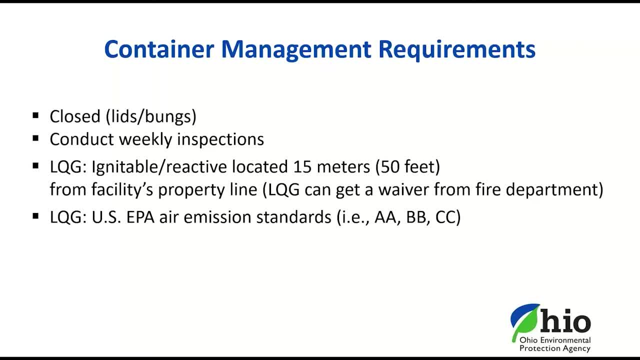 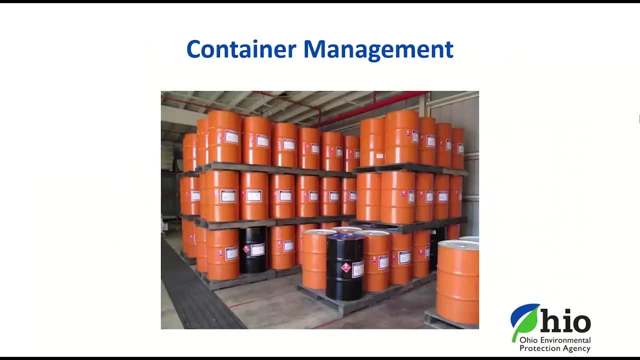 make sure your ignitable or reactive hazardous waste is stored at least 50 feet from the property line, unless you have a waiver from the fire department, and you must also comply with the federal air emission standards. here's an example of good container management. you can see the drums. 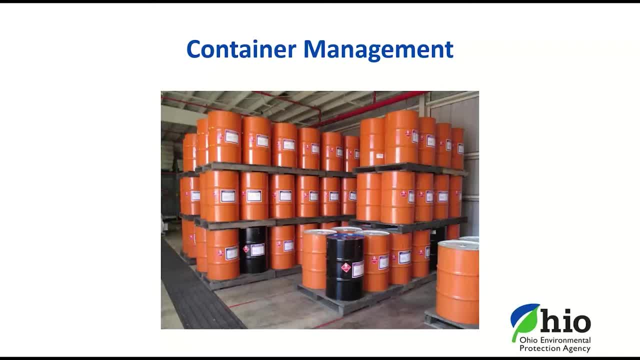 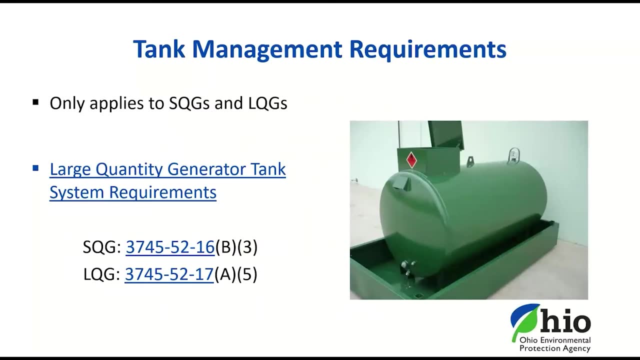 are labeled and closed. there appears to be dot labels on them indicating the contents are flammable and there are no signs of dents or leaks. now we are going to move into additional requirements for tanks. there are many requirements for large quantity generators who store hazardous waste and tanks, so the 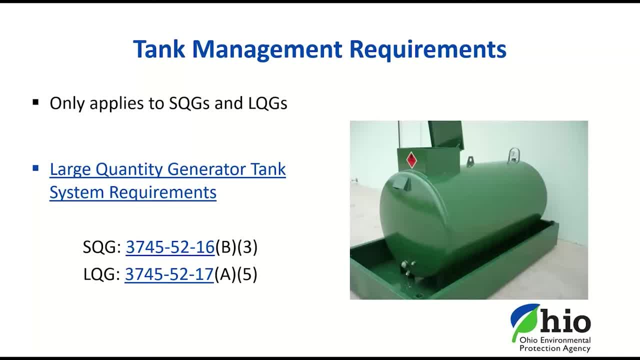 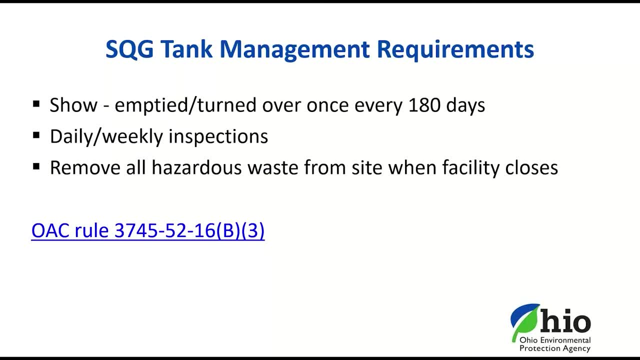 linked guidance document provides a lot of good information on that subject. for small quantity generators, you may accumulate hazardous waste in tanks for up to 180 days, or if you're transporting a distance of 200 miles or more, you can store the waste for up to 270 days. 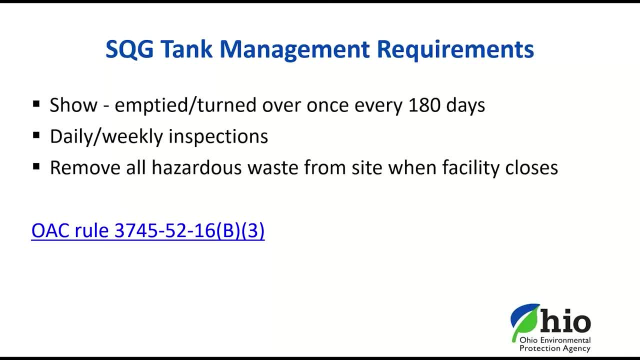 without a permit, as long as you never accumulate more than 13 200 pounds on site at any time on a daily basis. you need to inspect discharge control equipment, such as waste feed cutoff systems, bypass systems and drainage systems. inspect data gathered from monitoring equipment, such as pressure and temperature gauges, and inspect 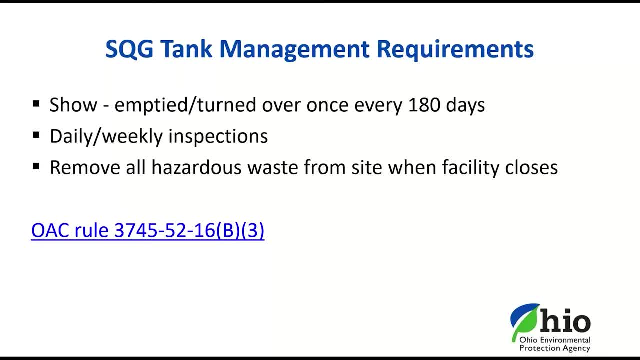 level waste in an uncovered tank. to ensure compliance with the tank freeboard requirements on a weekly basis, you need to inspect tanks to detect corrosion or leaking of fixtures or seams and inspect the area immediately surrounding the discharge confinement structures such as bikes or secondary containment for obvious signs of leakage. 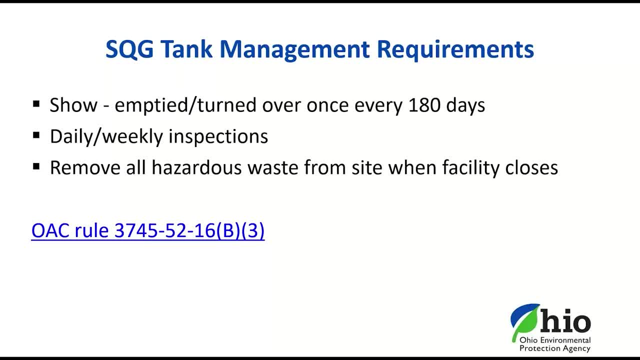 Upon closure of the facility, hazardous waste must be removed from the tank, as well as from discharge control equipment and from discharge confinement structures. Since the regulations for large quantity generators storing hazardous waste in tanks are lengthy, I've listed just a brief summary of the requirements on the slides. 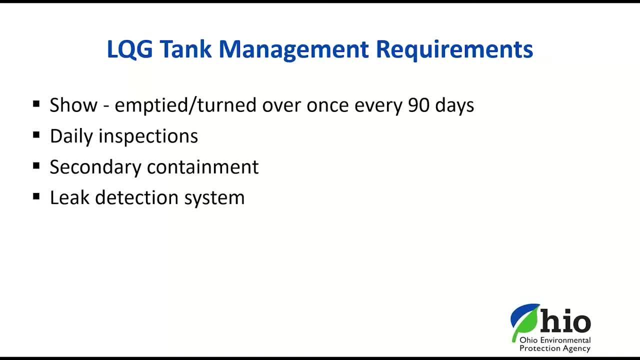 There need to be inventory logs or monitoring equipment to demonstrate tanks are turned over in the 90-day time frame. The tanks need to be inspected daily to identify leaks, deterioration, corrosion or structural fatigue in any portion of the tank or system components. 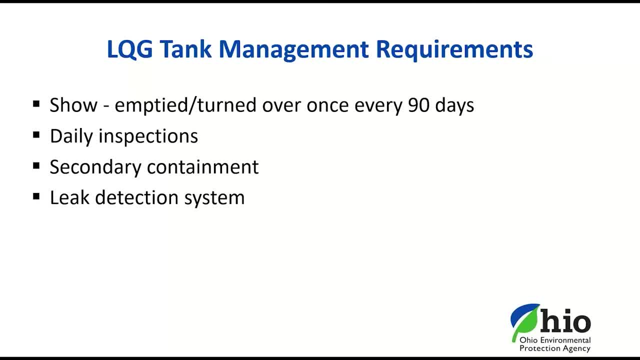 They also need to be equipped with secondary containment and leak detection systems to allow for detection of leaks from the primary or inner tank, while providing a secondary barrier. The tanks need to be equipped with secondary containment and leak detection systems to allow for detection of leaks from the primary or inner tank. 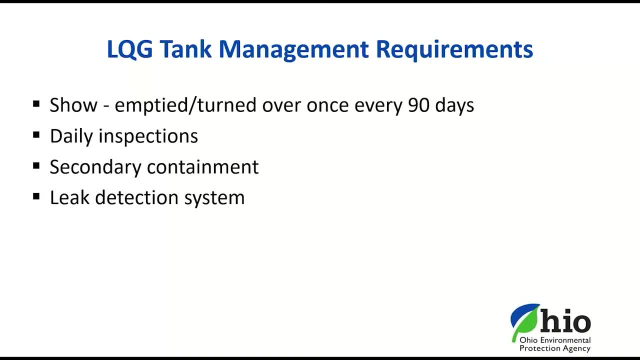 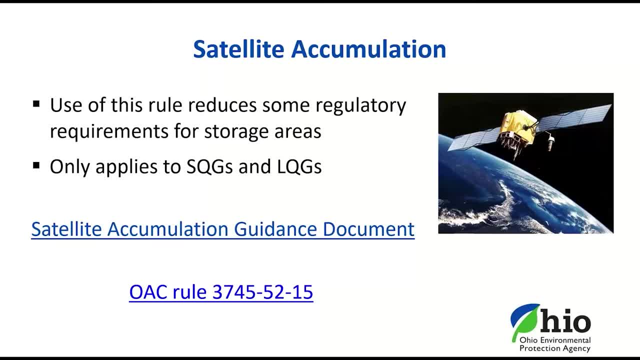 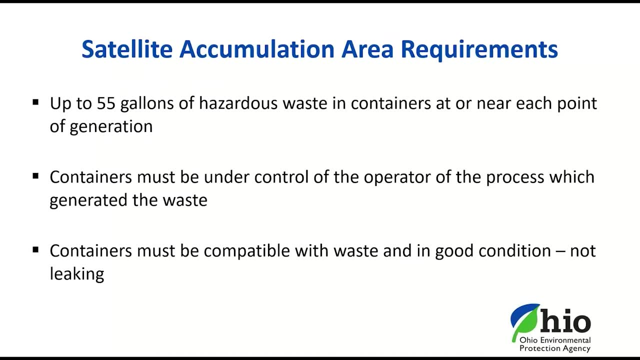 The tanks need to be certified by a professional engineer Upon closure of the facility. hazardous waste must be removed from the primary or inner tank, as well as from discharge confinement structures. The K Samuel nor can only have up to 55 gallons of hazardous waste per area, or 1 quart of acute 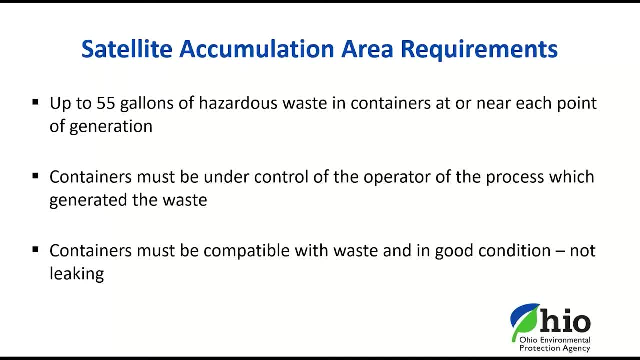 hazardous waste. The container must be located at or near the the point of generation. The container must be located at or near the point of generation under the control of the operator of the process that is generating that waste. This will hopefully prevent the addition of incompatible waste into the satellite container. 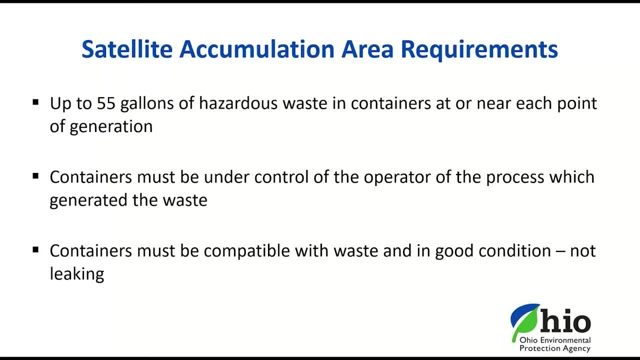 and prevent untrained personnel from coming into contact with the waste. The containers used to store waste need to be compatible with the contents. For example, you wouldn't want to store sulfuric acid in an unlined steel drum. that could cause it to corrode. 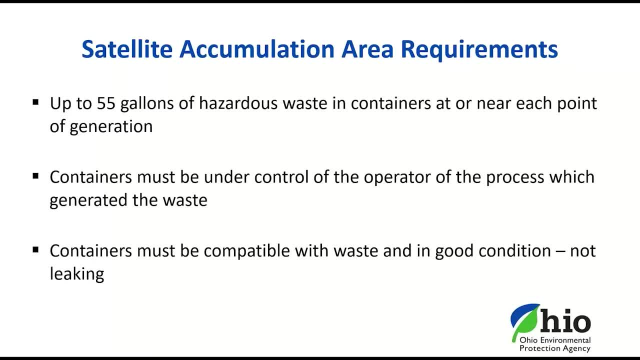 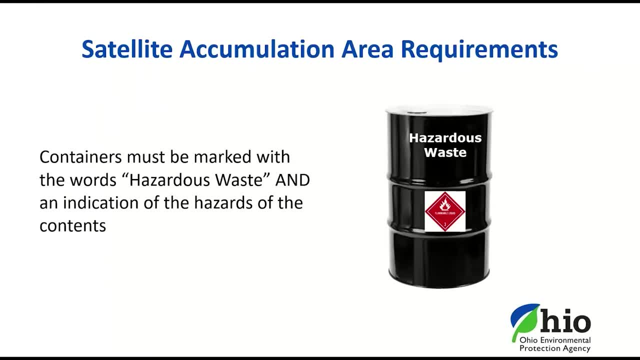 And the containers need to be in good condition, so there should be no dents, bulges or leaks. Marking and labeling requirements do apply to satellite containers, so they need to be labeled as hazardous waste and have an indication of the hazards of the contents. 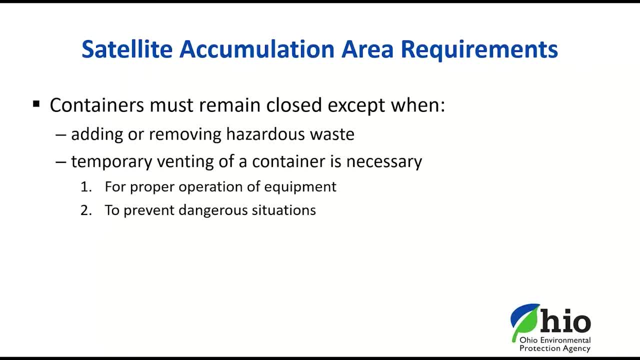 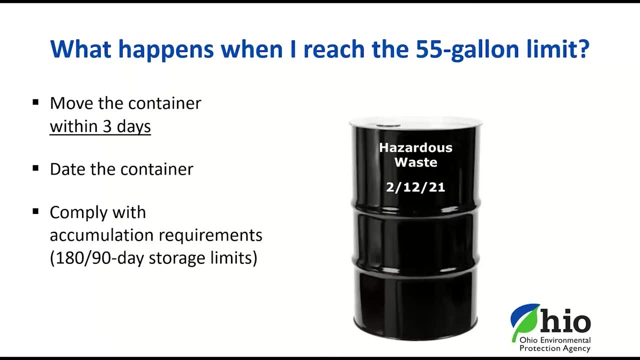 The satellite containers need to be kept closed except when actively adding or removing hazardous waste, Unless it is necessary to temporarily vent the container. Once the satellite container is full, you need to date it and move it to the central accumulation area within three calendar days. 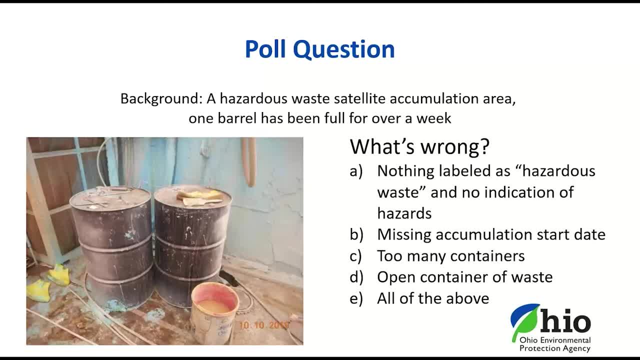 All right, it's time for our second poll question. Can you spot the violations that an inspector could cite for this satellite accumulation area where one barrel has been full for over a week? Okay, Thanks, Helen. The actual correct answer is all of them. 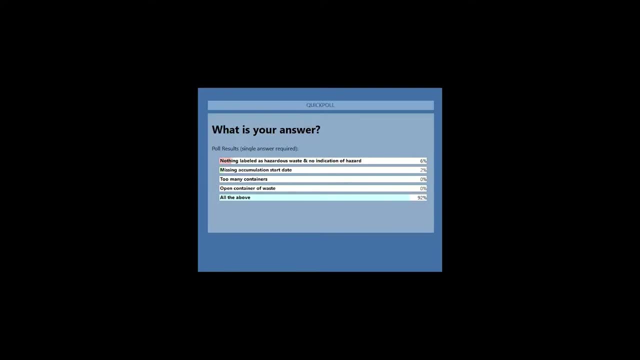 The bucket is open and it needs to be closed if the operator is not adding materials to it. Everything should have a label on it and if the barrel is full and at 55 gallons, it needs to be moved to the central accumulation area in three days or reaching to 55 gallons. 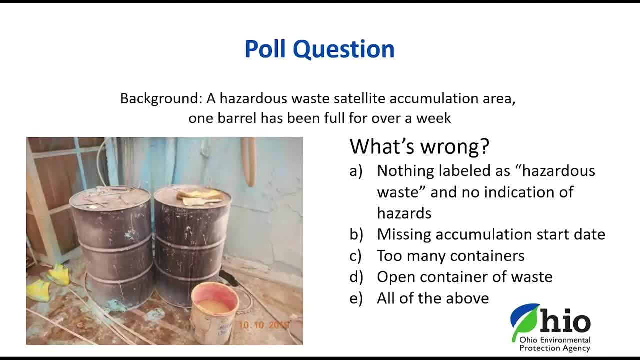 So with that detail in this example there are too many containers. If the barrel is full and at 55 gallons, it needs to be moved to the central accumulation area in three days. So with that detail in this example there are too many containers. 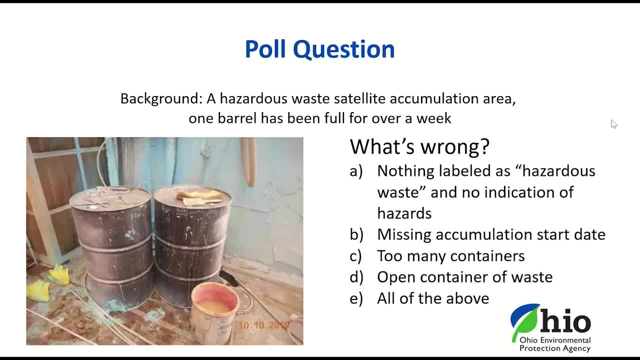 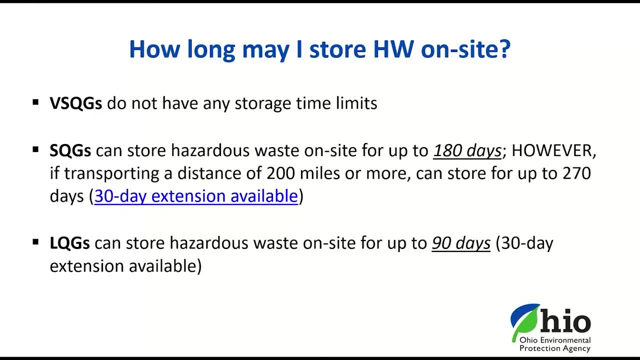 So, now that you have moved your waste to your central accumulation area, if you are a small quantity generator or a large quantity generator, you are limited in the number of days you can store it. Very small quantity generators don't have any storage time limits, but keep in mind: 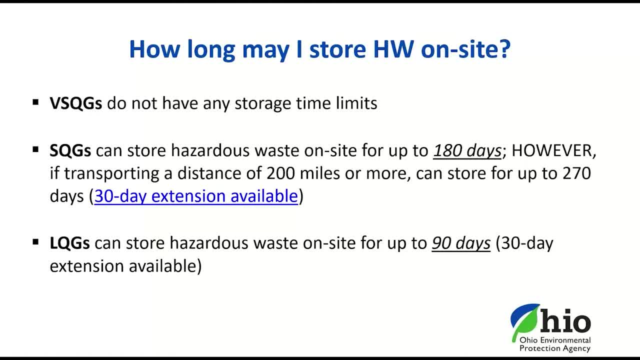 if you accumulate more than 2,200 pounds of hazardous waste on site at any one time, you become subject to the small quantity generator requirements until it's shipped off For small quantity generators. if you accumulate waste for longer than 180 days or 270 days. 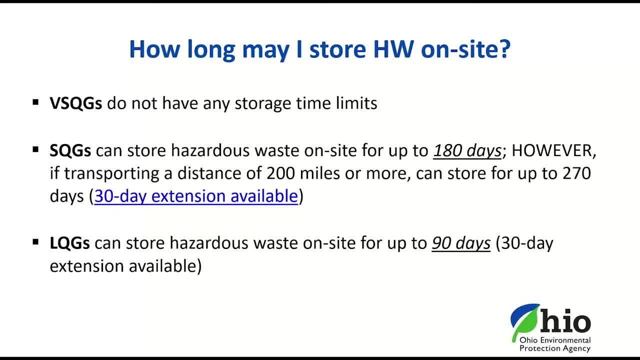 of transporting more than 200 miles, you must get a hazardous waste permit For large quantity generators. hazardous waste may not be accumulated at the central accumulation area for more than 90 days. Large quantity generators must maintain strict compliance with the 90-day timeframe since. 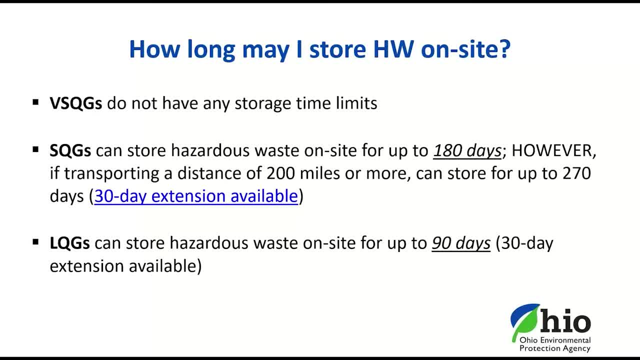 exceeding the allowable accumulation period can cause a generator to potentially be classified as an operator of an illegal hazardous waste storage facility. If you encounter unforeseen, temporary and uncontrollable circumstances, getting hazardous waste transported offsite before the deadlines, it's possible to obtain a temporary or uncontrollable. 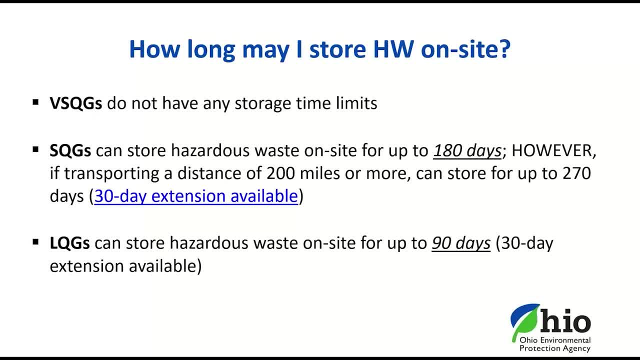 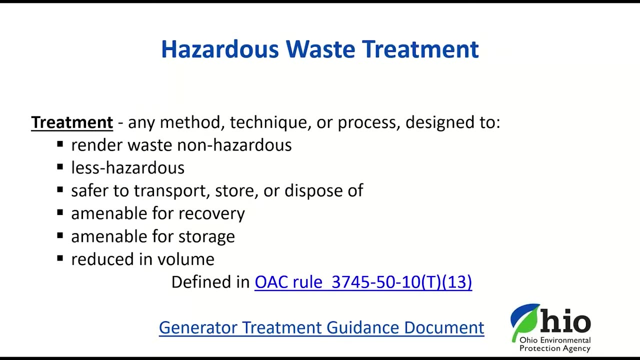 extension of 30 days through the accumulation provisions provided by the Director of the Ohio EPA. Contact the Ohio EPA to request an extension prior to the 90,, 180, or 270-day requirement. Generators may want to treat their hazardous waste on site for a variety of reasons, including. to render it less hazardous and to reduce Chroma or other damage. I would like to remind all generators that their hazardous waste is now on-site and that the next time you are in an area of bulk material, you will need the help of a generator. 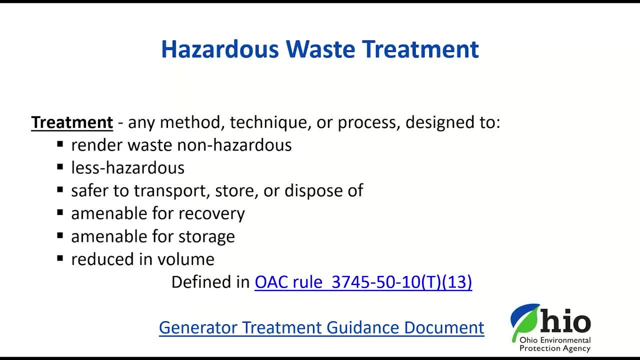 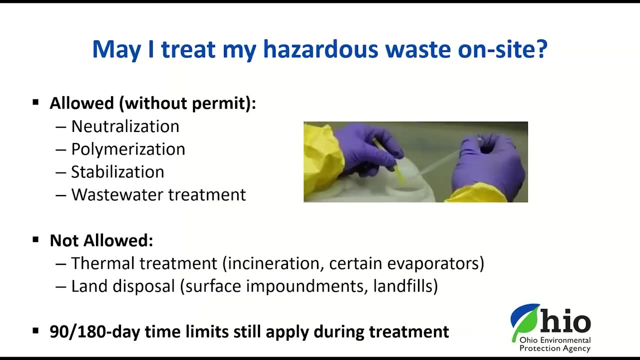 this make it easier to recover, store or transport or even reduce the volume. it's important to understand what is permissible for you to do as a generator. i've linked a guidance document with a lot more information. this is something you're considering at your facility. in general, there are 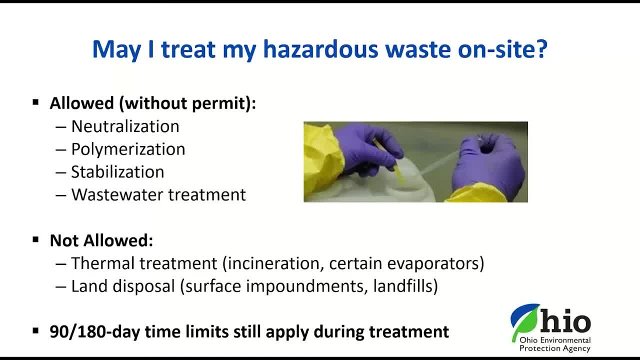 a few types of treatment that are allowed. you can perform neutralization, polymer polymerization, stabilization and wastewater treatment. treatment must be done in tanks, containers, on drip pads or in containment buildings, and you are not allowed to conduct any thermal treatment or land disposal without a permit. also, keep in mind that the 90 or 180 day storage 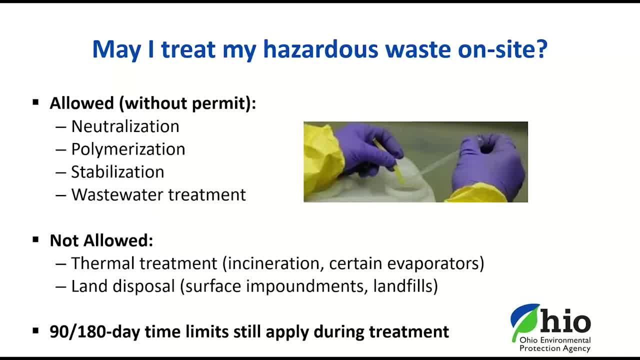 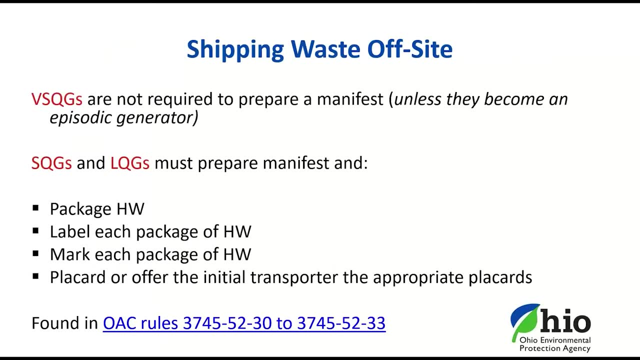 time limit still applies while you are treating your hazardous waste. it is always a good idea to reach out to us if you have any questions before you treat your hazardous waste. once waste has reached the accumulation limit, it's time to ship it off-site, and there are some specific shipping requirements that you need to that need to be followed- very small. 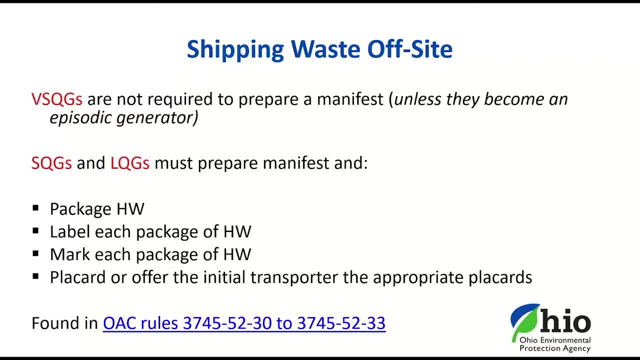 quantity generators aren't required to prepare a manifest, unless that waste was generated from a episodic event. however, if you are shipping 2200 pounds or more hazardous waste, you would then be a small quantity generator. small quantity generators and large quantity generators must prepare a manifest before shipping hazardous waste off-site. 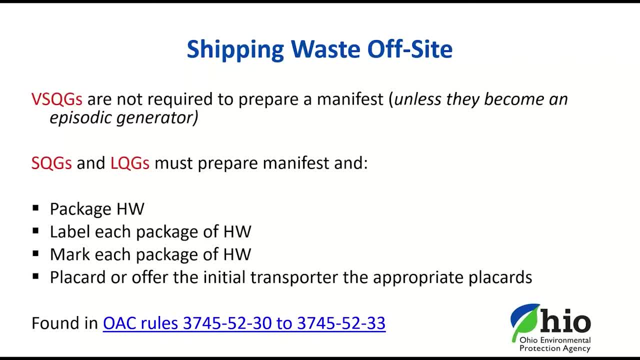 transporting hazardous waste off-site also has us department of transportation requirements. the hazardous waste being transported needs to be packaged correctly as required by us department of transportation regulations 49 cfr, parts 173, 178 and 179.. the material needs to be labeled and marked. 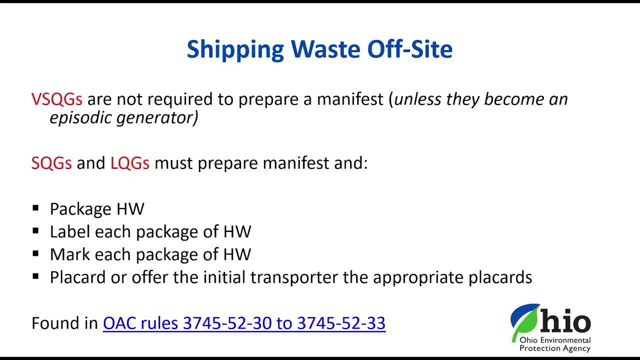 as defined in 49 part 172, and before you have the hazardous waste transported off-site, you must placard or offer the initial transporter the correct backwards for the material. if you have any specific questions or thoughts, please write a comment and we will look at each. 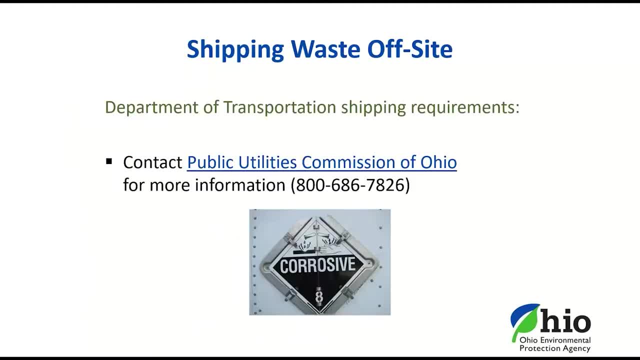 question in detail as well. remember to check your auspicesㅋㅋㅋㅋ cookie. the qab will be shown down by the link chose the specific frρι buenos dias vale in commờ- to youtube. that's alontad, it's free and you can visit jupytersupplycom and if you have any questions or 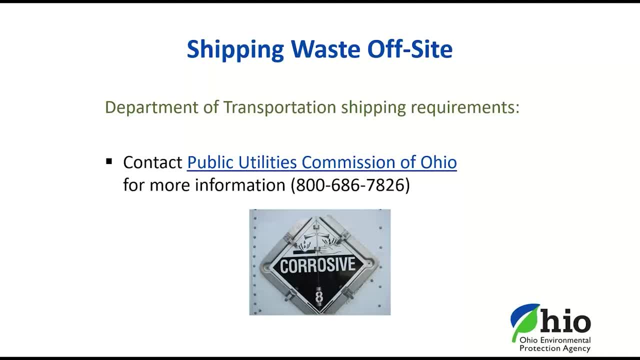 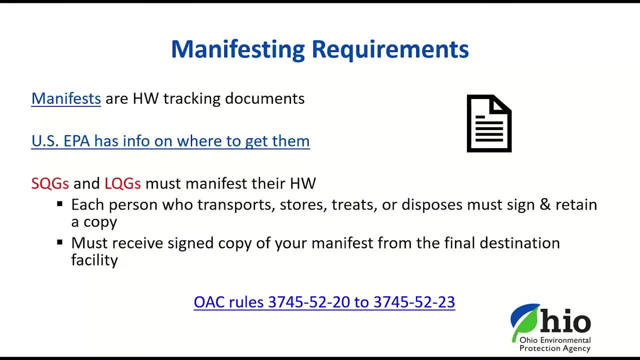 questions regarding DOT shipping requirements, you can contact the Public Utilities Commission of Ohio. They oversee these regulations in Ohio. Manifests are multiple copy tracking documents that accompany hazardous waste shipments. The manifest acts as a chain of custody for the waste from the point it leaves your business. 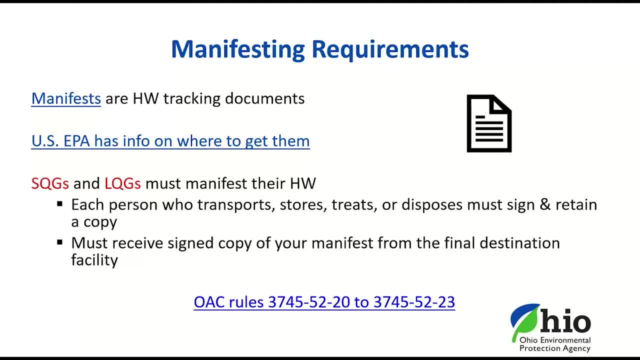 until it reaches its final destination. Each person who generates, transports, stores, treats or disposes of waste must sign and retain a copy of the manifest. This provides a traceable link between your business and the designated facility. Once the hazardous waste reaches its final destination, the person receiving your waste returns a signed copy. 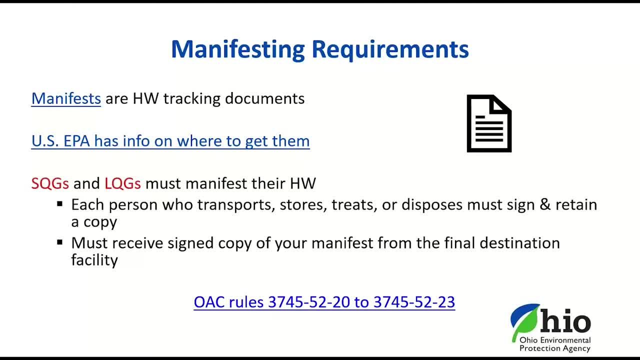 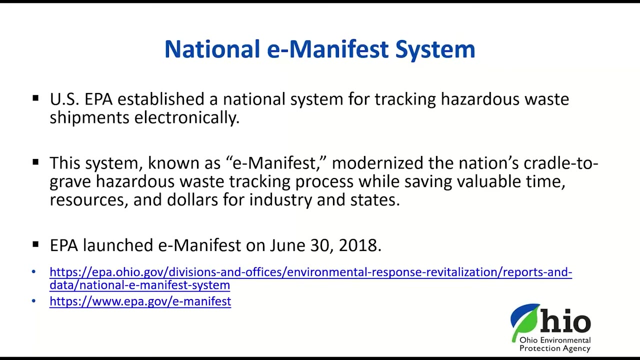 of the manifest to you. Be sure to provide enough copies of your manifest so that each transport has a copy for their records. The designated facility must have two copies: one for their records and one that is returned to you. In 2018, US EPA launched the eManifest system. 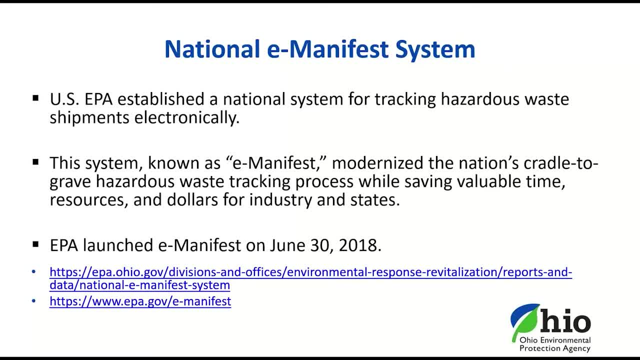 which is a national electronic system to track hazardous waste shipments. Many of you may already be using eManifest instead of paper copies at this point. If you aren't, then you should know that there is no history of anetta. Now you know the meaning of eManifest. 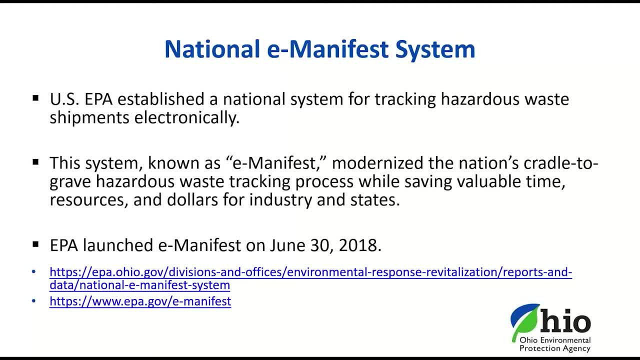 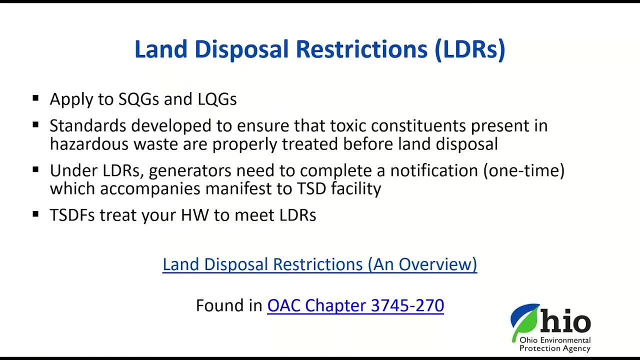 in English, so let me show you what you can do with that. Check the website for more information. It is full of information, including a video and instructions on how to sign up for the service. LDRs. LDRs and US EPA intended that land disposal restrictions would ensure that the toxic constituents 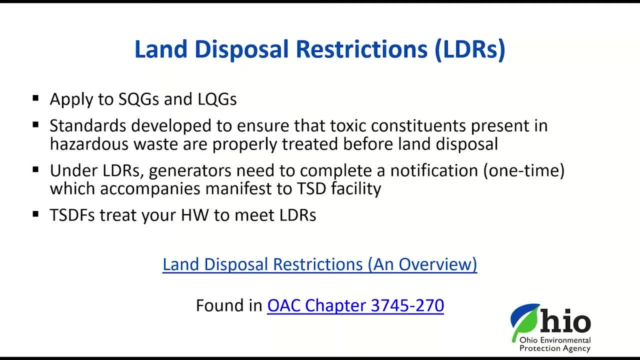 present in hazardous waste are properly treated before the waste is land-disposed. Hazardous waste can still be admitted to the government after disposal is completed. US EPA also. Hazardous wastes, or some component of them, are often placed into permitted hazardous waste. 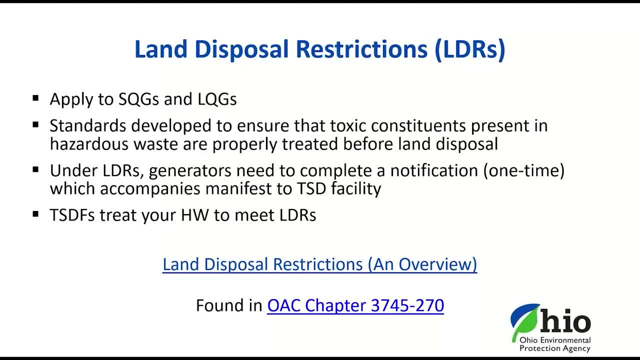 landfills. The disposal of this waste in a landfill has the potential, over a long period of time, to threaten human health and environment by leaking hazardous constituents into the groundwater, even though the landfill has a liner and other safeguards. As a result, most hazardous. 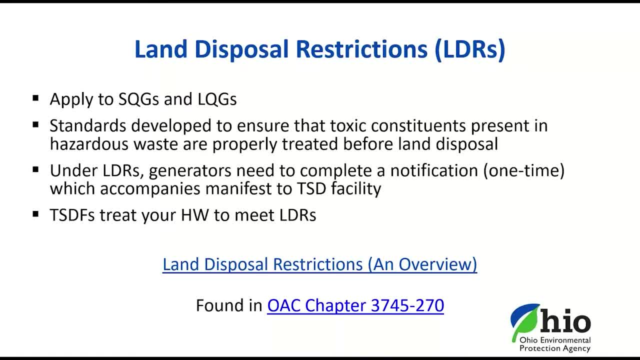 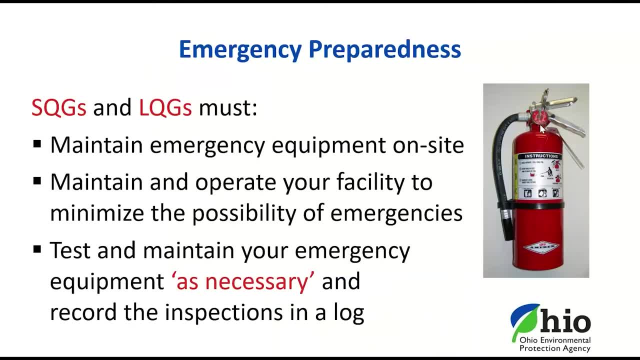 wastes must be treated to meet specific treatment standards prior to disposal in a permitted hazardous waste landfill. Now we're moving into the requirements for emergency preparedness. There are no prescribed emergency preparedness requirements for very small quantity generators. Small quantity generators and large quantity generators are not required for emergency preparedness. 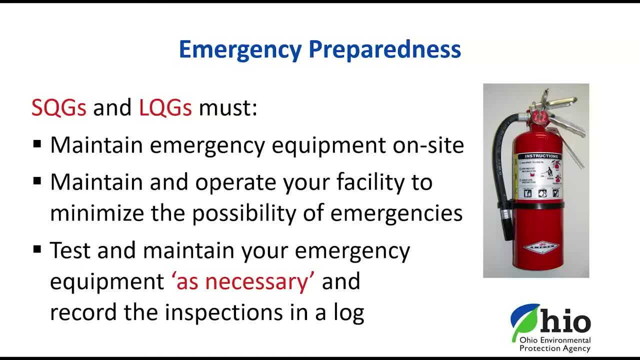 Small quantity generators are required to maintain emergency equipment on site. The type of emergency equipment is going to vary based on your facility, but the common ones include fire extinguishers, alarm or communication systems, spill kits, personal protective equipment and decontamination equipment. The testing frequency is also going to vary and is typically based on. 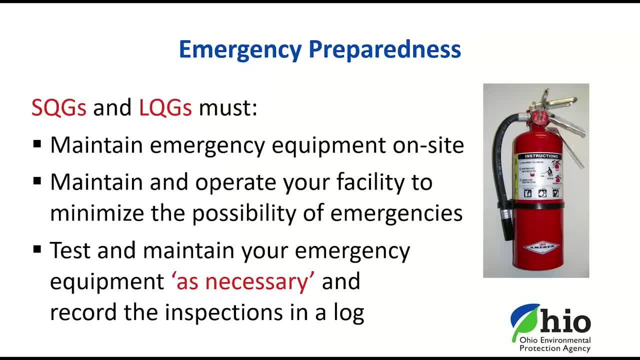 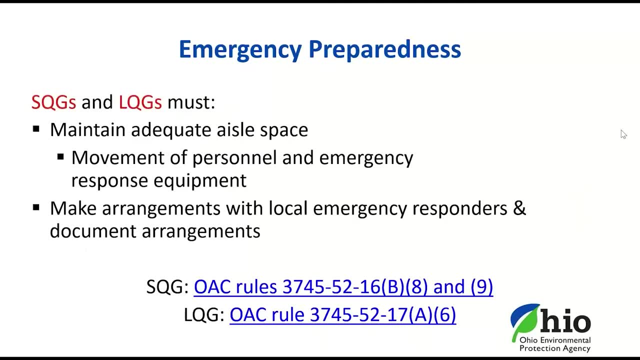 manufacturer's recommendation and common sense, especially when it comes to spill kits. Some may be used more frequently, So you'll want to inspect them at appropriate intervals to ensure that you have adequate and functional supplies. As part of emergency preparedness, it's necessary to maintain adequate IO space. Having IO 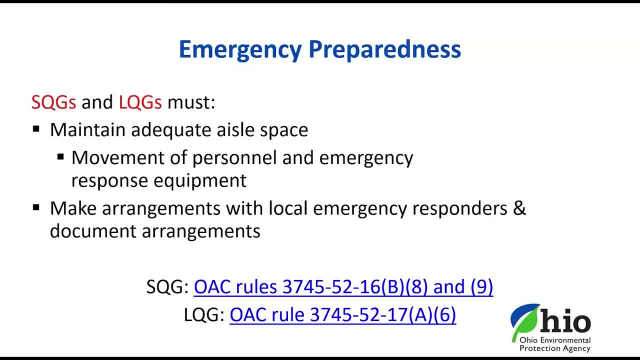 space to be able to read the labels is great, but the important thing is the space is required so that personnel and equipment can get in and respond to a fire. Small quantity generators and large quantity generators are also required to make arrangements with local emergency authorities and keep documentation that arrangements have. 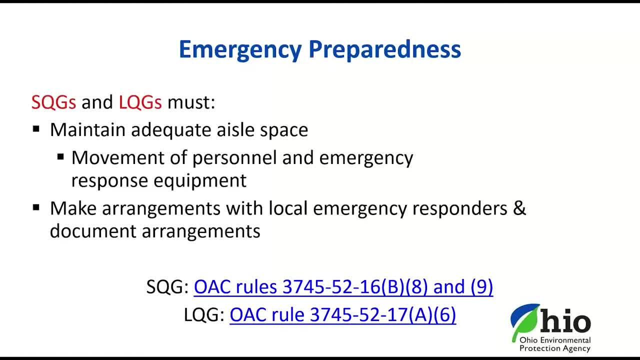 been made or document the failed attempts to make arrangements. The purpose of working with local responders is to help them be familiar with your facility so they know the layout, the properties of the hazardous waste on site where people are likely to be working and. 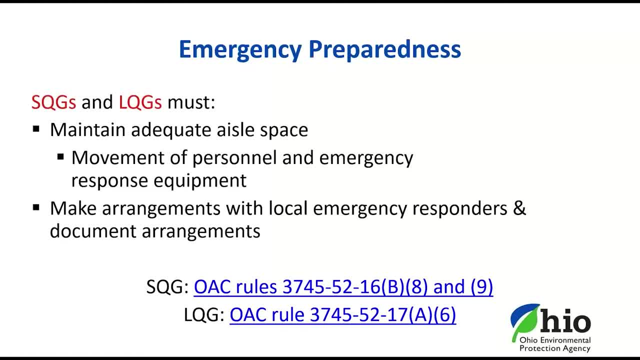 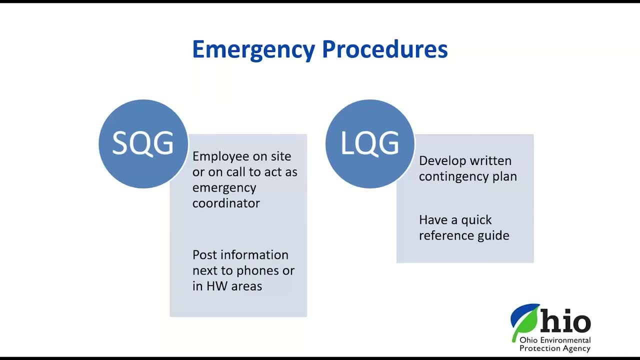 possible evacuation routes. The purpose of working with local responders is to help them make decisions on the location of evacuation routes. All of these details are necessary if they ever need to respond to an emergency. If you are a small quantity generator, you must have at least one employee on the premises. 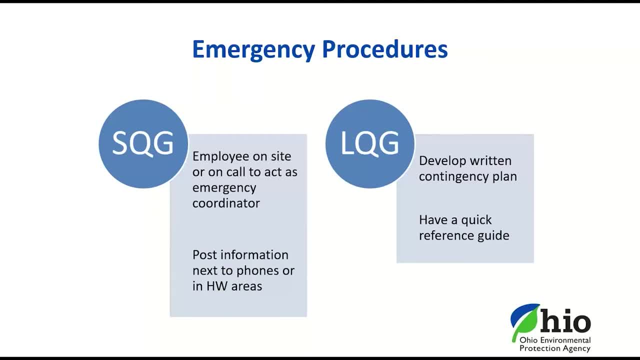 or on call who can respond to all emergencies at the facility. That person should be able know that, to call the fire department if there is a fire or attempt to extinguish a fire using a fire extinguisher, to contain and clean up spills as soon as practical and if you have a fire. 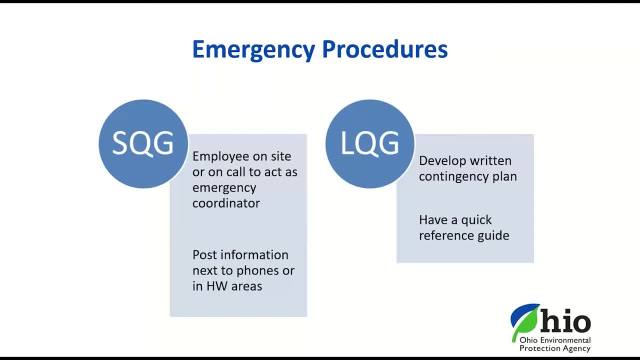 explosion or other release that could threaten people outside of your facility, or if the spill has reached surface water, then you must immediately notify the national response center at 1-800-424-8802. when posting information, include the name and emergency telephone number of the emergency. 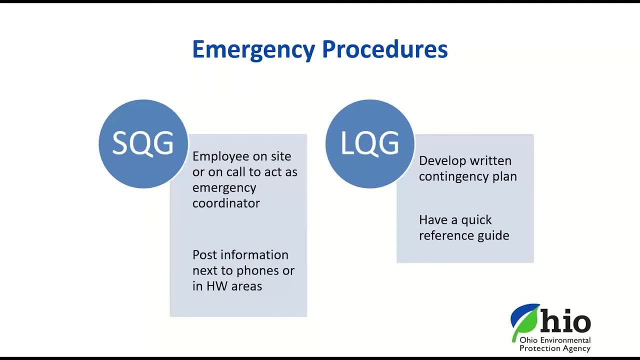 coordinator, the location of fire, extinguisher, extinguishers and spill control material and, if present, the fire alarm and the telephone number for the fire department, unless the facility has a direct alarm. if you are a large quantity generator, you must prepare and maintain a written contingency plan. the plan must be designed to minimize the risk to the fire department. 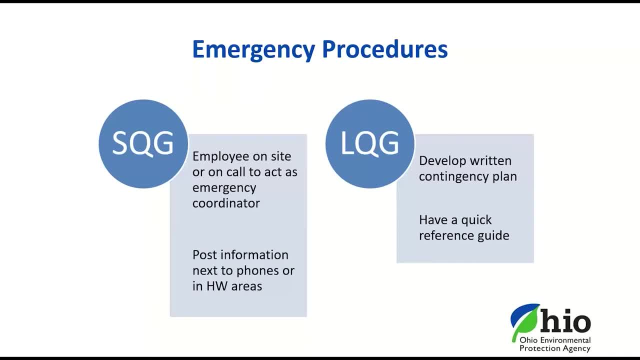 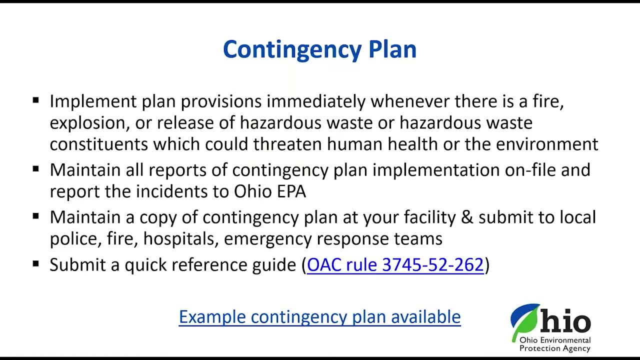 minimize hazards, to minimize hazards to human health or the environment from fires, explosions or any unplanned, sudden or non-sudden releases of hazardous waste, and the plan needs to be implemented immediately- immediately in those cases. in addition, a large quantity generator must maintain all reports of contingency plan implementation on file. 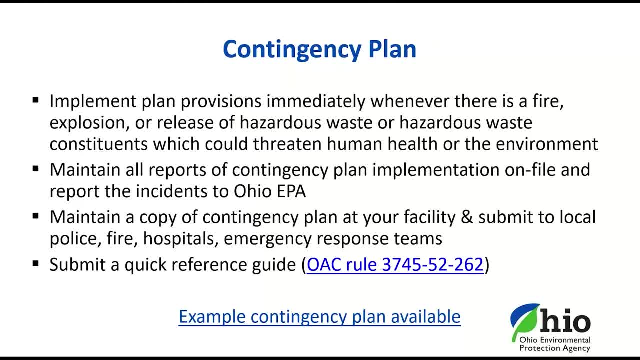 and report these instances, instances and incentives to the director of ohio epa. a copy of your contingency plan and revisions must be maintained at your facility and submitted to all local police, fire departments, hospitals and emergency response teams. here's a link to our generator handbook and in appendix 3, 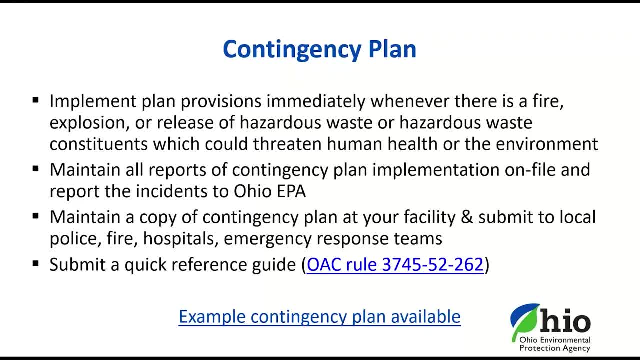 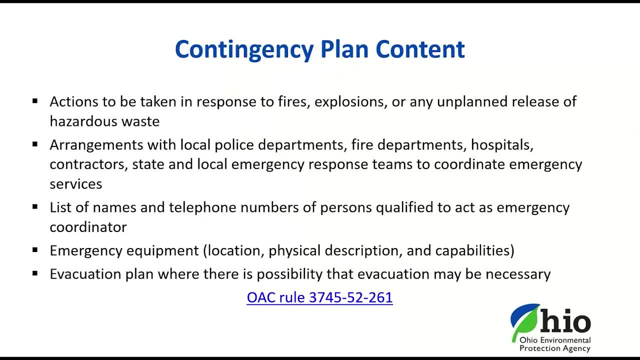 there is a sample contingency plan for your reference. the items that are required to be included in the contingency plan are outlined in a role 52-61. the plan needs to specify the actions that need to be taken when responding to fires, explosions or releases of hazardous waste. it needs to describe the arrangements with the local. 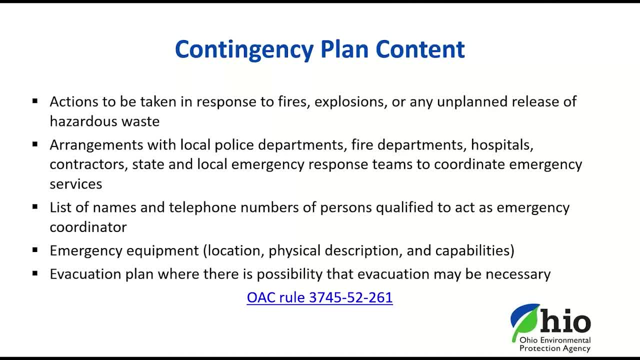 emergency responders and have a list of names and telephone numbers of all emergency coordinators. the plan needs to list all emergency equipment and include the emergency equipment that is required to be included in the contingency plan. the plan also needs to provide details such as their location, description and explanation of. 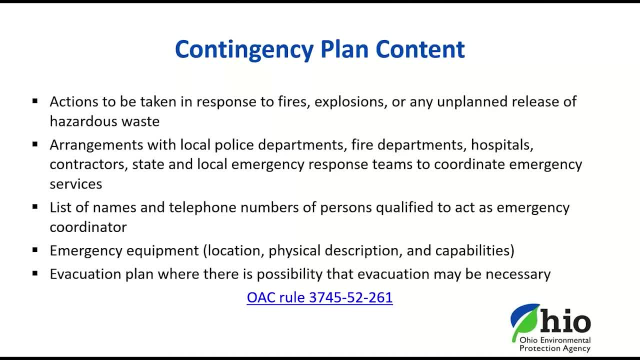 capabilities. and, finally, the contingency plan needs to include an evacuation plan where there is a possibility that an evacuation might be needed. evacuation plan needs to include details such as the signals used to begin evacuation, evacuation routes and alternative evacuation routes in case in cases where a primary route could become 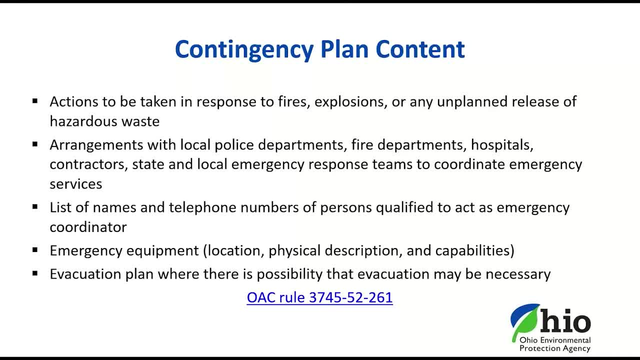 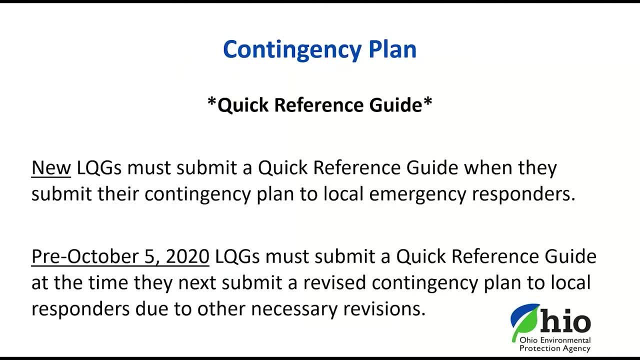 blocked or release of hazardous waste or a fire. Along with the contingency plan, large quantity generators are required to have a quick reference guide to provide easy access for emergency responders to the most critical information when responding to an emergency. New facilities need to submit this quick reference guide when they are submitting their plan. 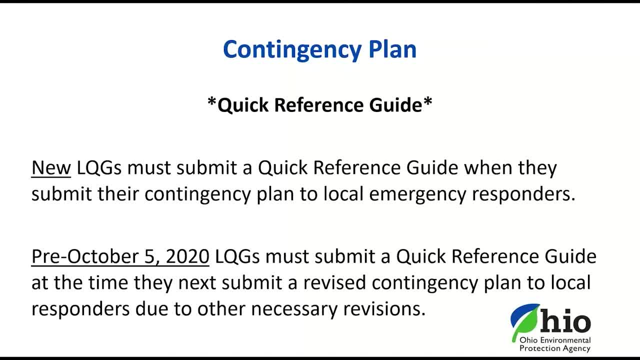 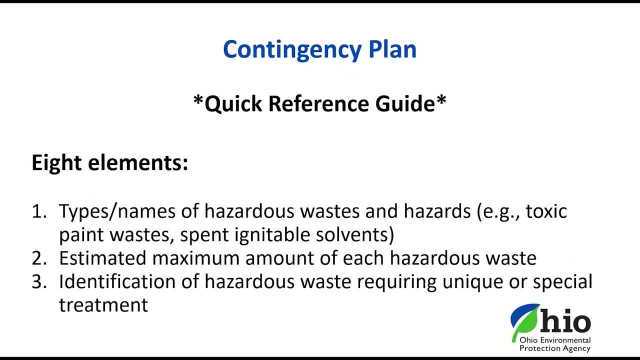 But large quantity generators that were registered prior to October 5, 2020 only need to submit the quick reference guide when they submit a revised plan or other necessary revisions. The quick reference guide consists of eight elements. It needs to list the types of hazardous waste and their associated hazards. the estimated 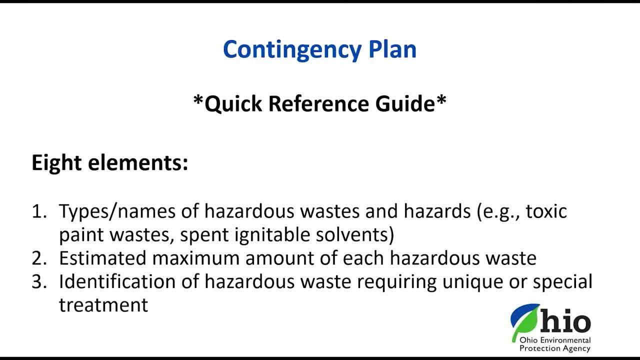 maximum amount of each hazardous waste on site and specify if there are any hazardous wastes that require unique or special treatment, such as things that may react violently with water, because that's something the fire department would want to know about, or if you have something. 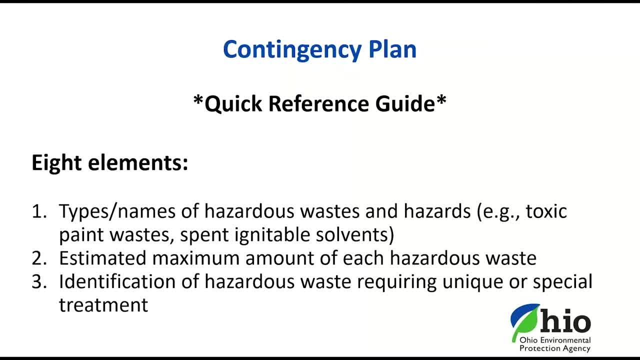 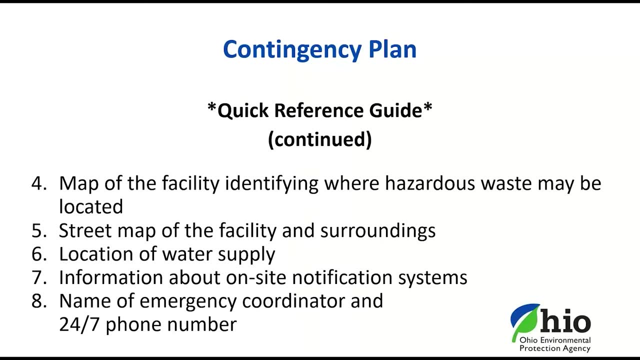 like hydrofluoric acid. that will dictate the type of PPE someone wears and how medical professionals will treat anyone that's exposed to it. The quick reference guide needs to include a map of the facility that shows where hazardous waste is located, and there needs to be a street map that shows the surrounding businesses. 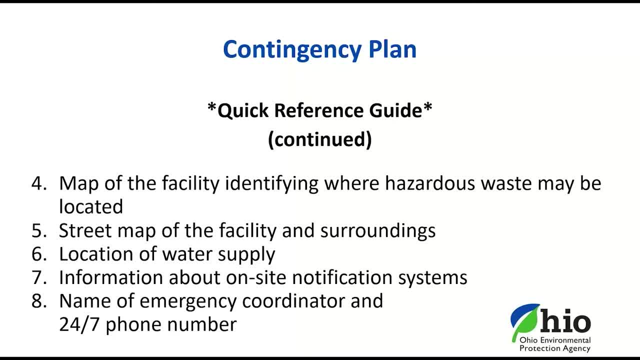 residents and schools. The location of the water supply needs to be identified and the information about on-site notification systems to communicate with the fire department. The quick reference guide needs to include a map of the facility that shows where hazardous waste is located and the information about on-site notification systems to communicate. 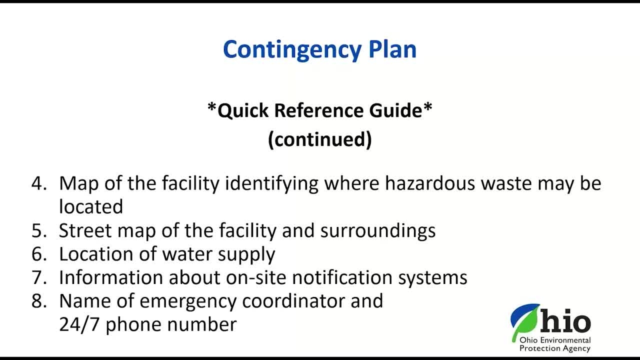 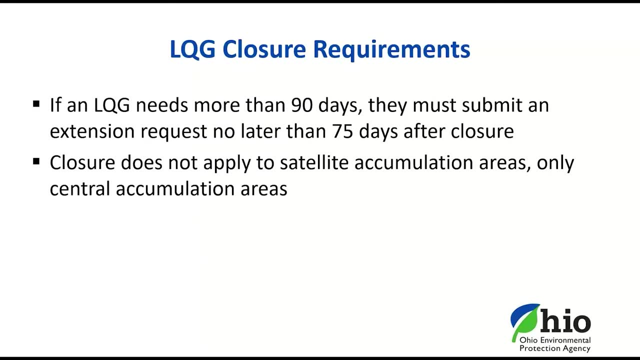 with facility personnel and the name and number of the person designated as the emergency coordinator. Now let's cover large quantity generator closure notification requirements. When an LQG closes either an accumulation area or the entire facility, the LQG must. a notification is required when closing an accumulation unit, including the central. 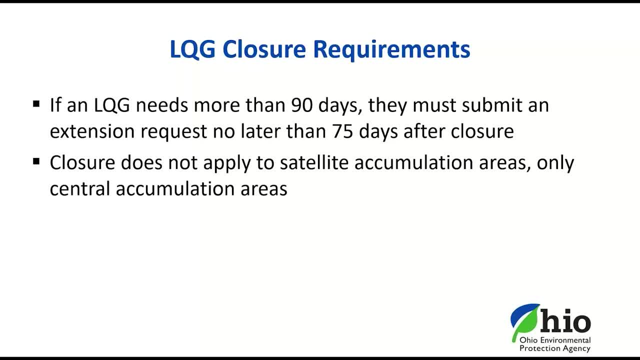 accumulation area. they need to either place a notice in the operating record within 30 days of closing it or they can notify the ohio epa within 90 days that the closure performance standards have been met. if the entire facility is closing, you will need to notify the ohio epa. 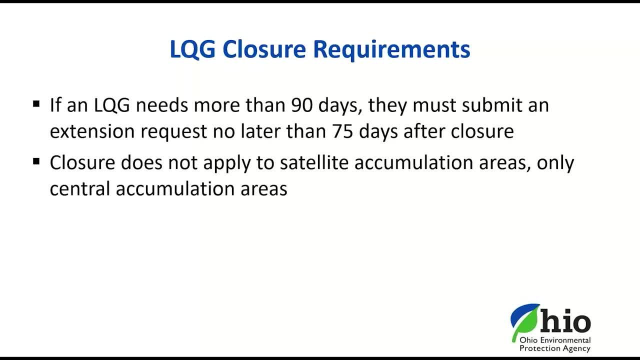 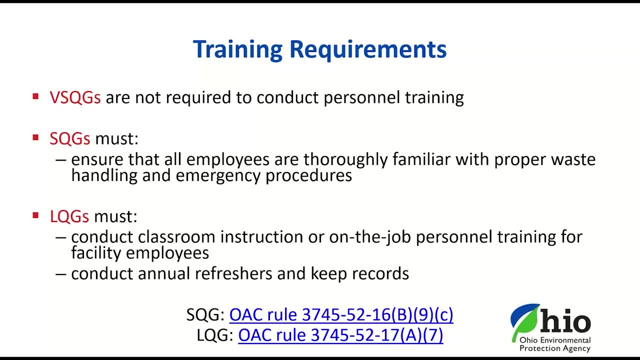 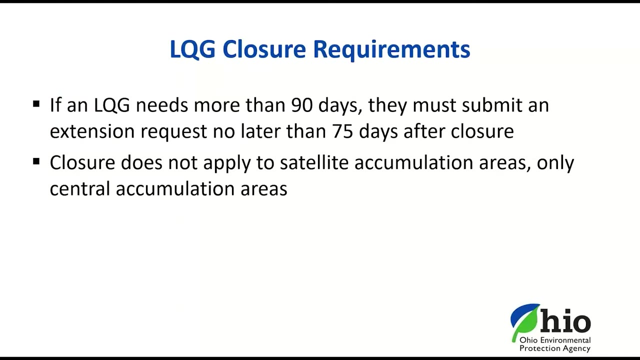 30 days prior to closing and then again 90 days after closing to confirm the closure performance standards have been met. if more than 90 days is needed to meet the closure performance standards, an extension can be requested, but keep in mind you would need to request it no later than 75 days after closing the facility. 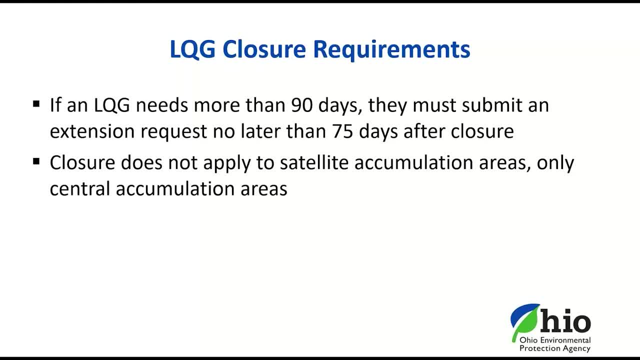 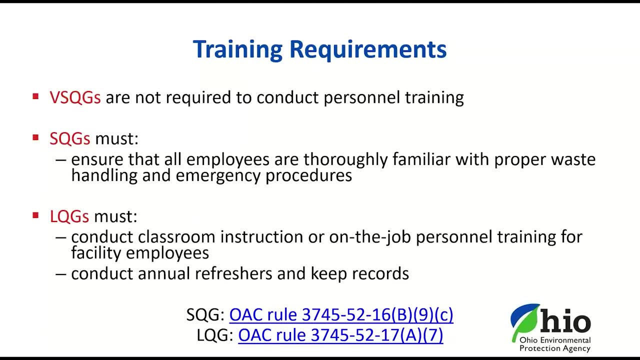 you can't wait until the last possible moment to ask for an extension. and just to clarify: closure is not needed for satellite accumulation areas. there are specific hazardous waste training requirements for small quantity generators and large quantity generators. small quantity generators must ensure that all employees are thoroughly familiar with proper waste handling and emergency. 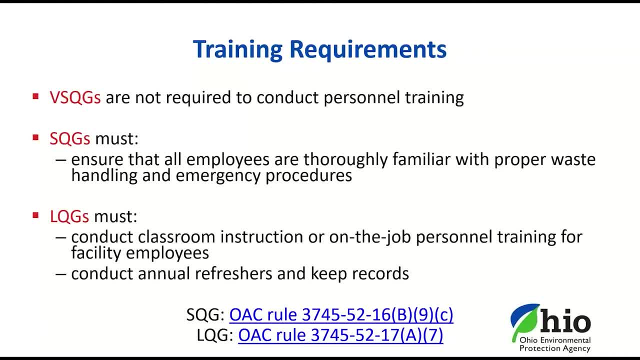 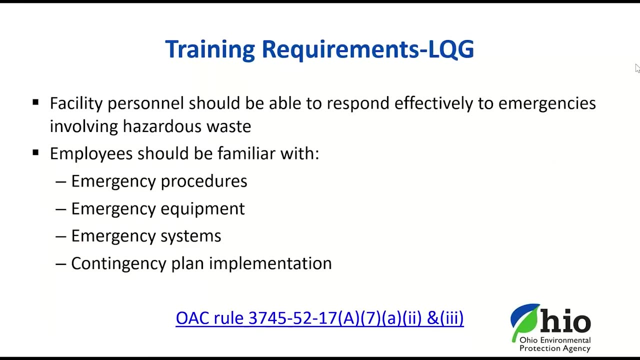 procedures relevant to their responsibilities during normal facility operation and emergency situations. this is a performance based training standard. large quantity generators must conduct classroom instruction or on the job training and maintain documentation. do Large quantity generators have more in-depth training requirements? Personnel involved with hazardous waste management should have training in proper waste handling. 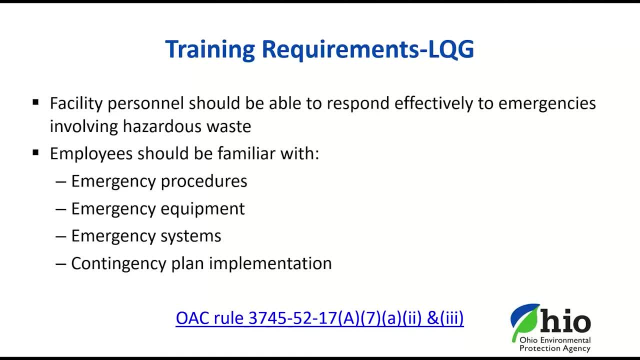 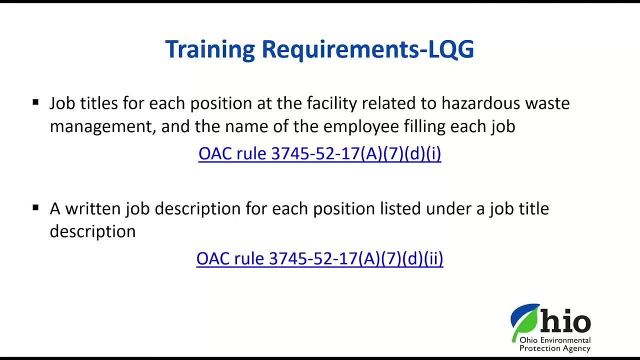 and emergency procedures appropriate to the types of waste managed. Generally, employees need to be familiar with the types of emergency equipment on site, the communication systems and how to implement the contingency plan. Specific information that needs to be maintained includes the job title and written job description. 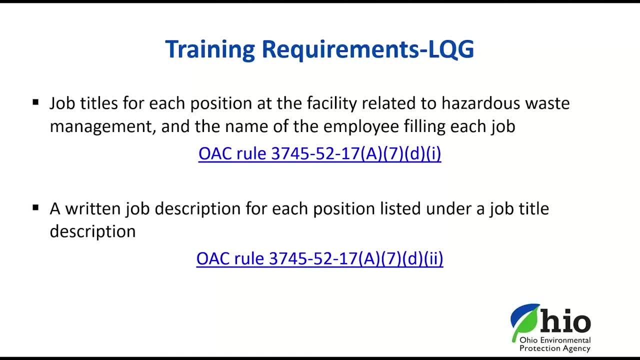 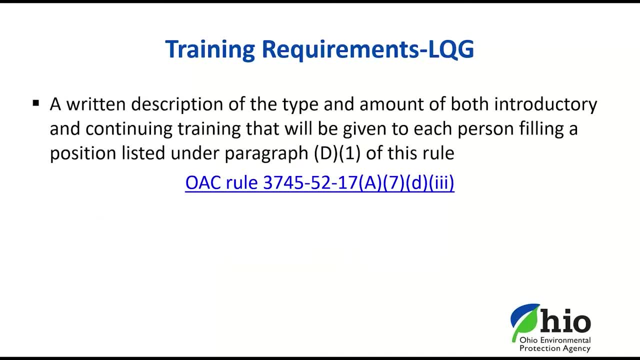 for each position related to hazardous waste management and the name of the employee filling that position. Facility personnel need to complete an initial training program within six months of being hired and participate in annual refreshers. There needs to be a written description of the type and amount of training that will. 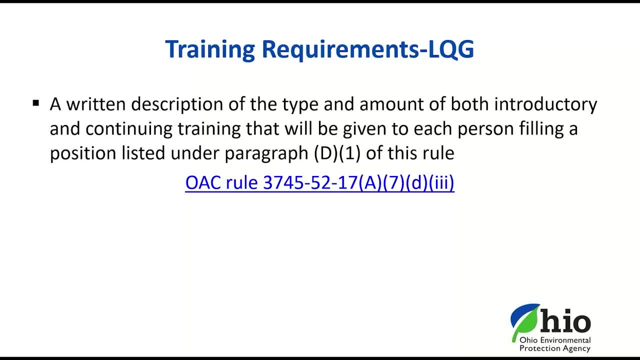 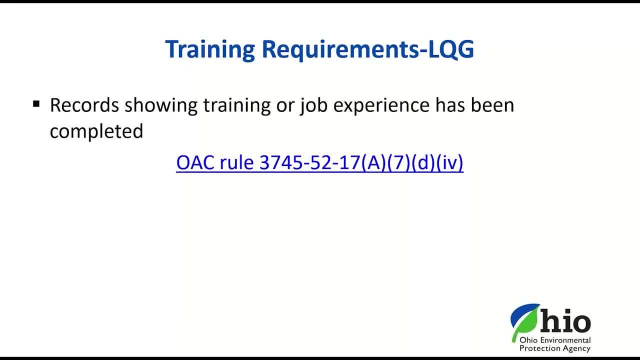 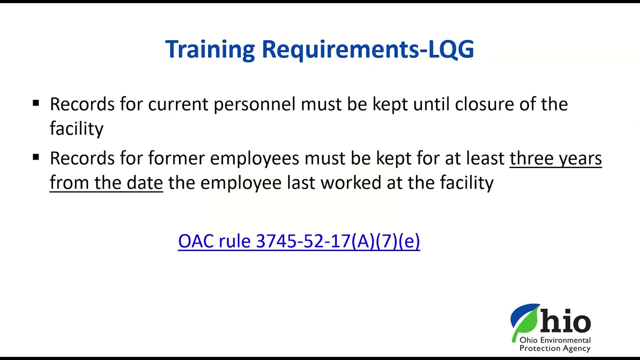 be given to each job position. There also needs to be some form of record kept to document the training. For example, a copy of the training sign-in sheet would be acceptable. Slide 8, Slide 9, Slide 10. Personnel training records on current employees need to be kept until the closure of the facility. 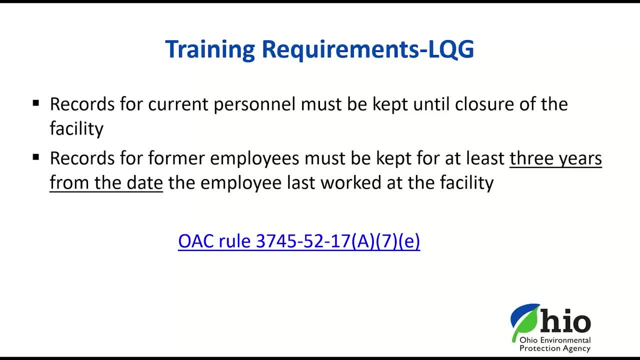 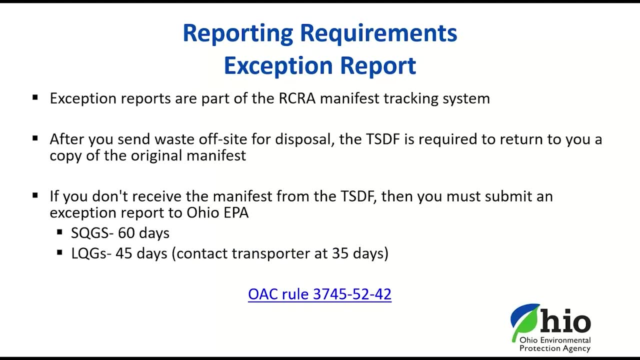 Personnel training records for former employees need to be kept for at least three years from the date the employee last worked at the facility. Slide 11. Now we are going to go over a few reporting requirements. An exception report is another element of the manifest tracking system. 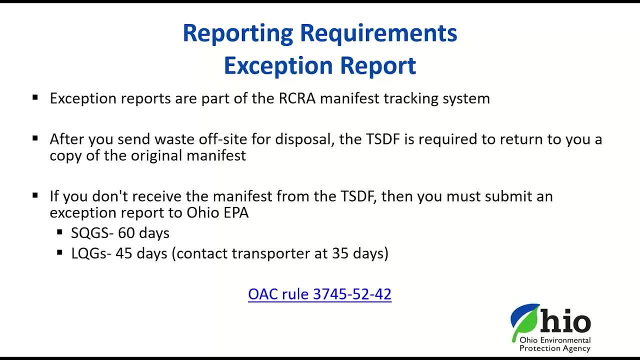 This report lets the Ohio EPA know that you didn't receive a signed manifest back in the appropriate timeframe. Small quantity generators need to submit this report if a signed manifest isn't received within 60 days, And large quantity generators need to contact the transporter and or TSDF to determine the 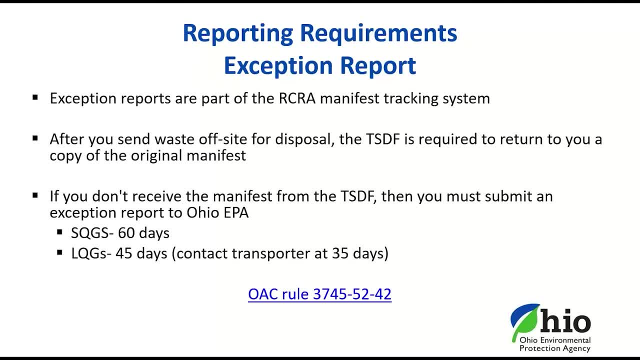 status of their waste. If a signed manifest isn't received within 35 days, a report needs to be submitted. If it's still not received within 45 days, a report needs to be submitted. Slide 11, Slide 12, Slide 13. 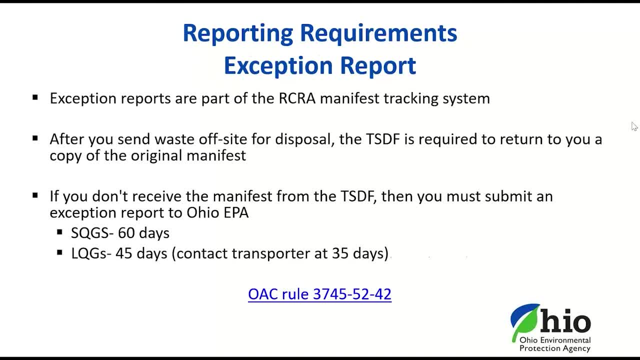 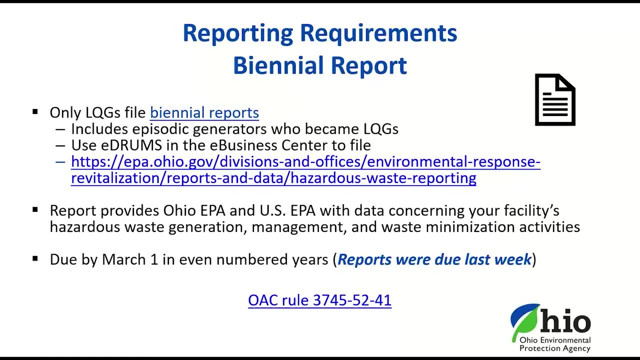 Slide 14, Slide 15, Slide 16, Slide 17, Slide 17, Slide 18, Slide 19, Slide 20, Slide 21, Slide 22, Slide 23, Slide 24, Slide 25, Slide 26, Slide 27, Slide 28, Slide 29. 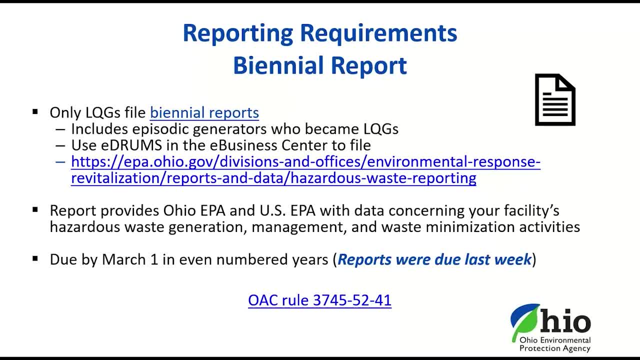 Slide 30, Slide 31, Slide 31, Slide 32, Slide 34, Slide 35, Slide 36, Slide 37, Slide 38, Slide 39, Slide 40, Slide 41, Slide 42, Slide 43, Slide 44, Slide 45, Slide 46. 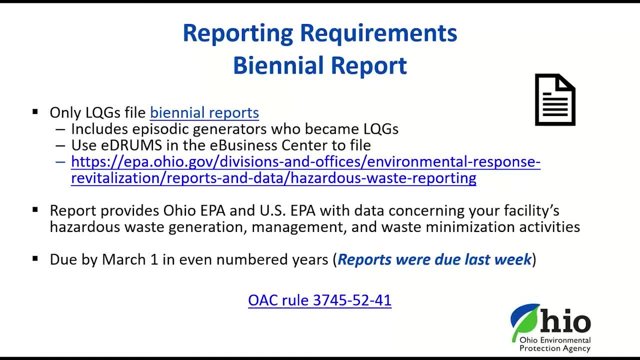 Slide 47, Slide 48, Slide 49, Slide 51, Slide 51, Slide 52, Slide 53, Slide 54, Slide 56, Slide 57, Slide 58, Slide 58, Slide 59, Slide 51, Slide 52, Slide 56, Slide 57. 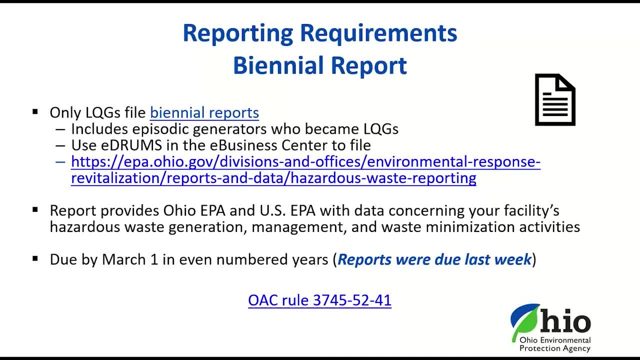 Slide 58, Slide 58, Slide 59, Slide 51, Slide 52, Slide 53, Slide 54, Slide 56, Slide 57, Slide 58, Slide 59, Slide 51, Slide 52, Slide 53, Slide 54, Slide 56, Slide 56. 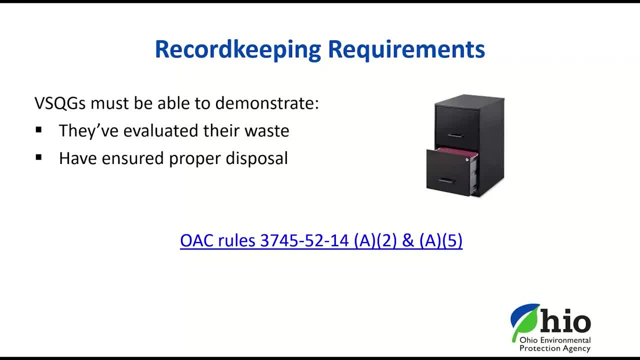 Slide 57, Slide 58, Slide 58, Slide 51, Slide 52, Slide 53, Slide 54, Slide 56, Slide 56, Slide 57, Slide 58, Slide 59, Slide 60, Slide 61, Slide 62, Slide 63, Slide 64. 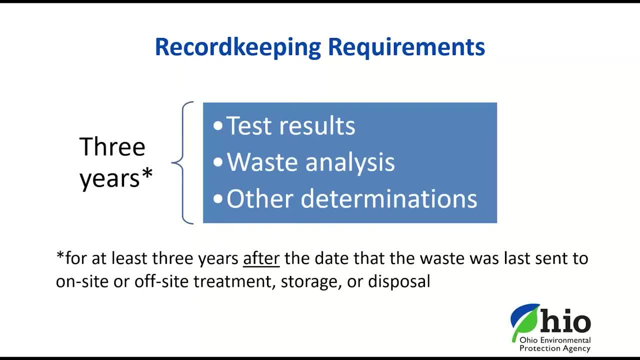 Slide 65, Slide 67, Slide 68, Slide 68, Slide 69, Slide 69, Slide 70, Slide 71, Slide 71, Slide 72, Slide 73, Slide 74, Slide 75, Slide 76, Slide 76, Slide 77, Slide 78. 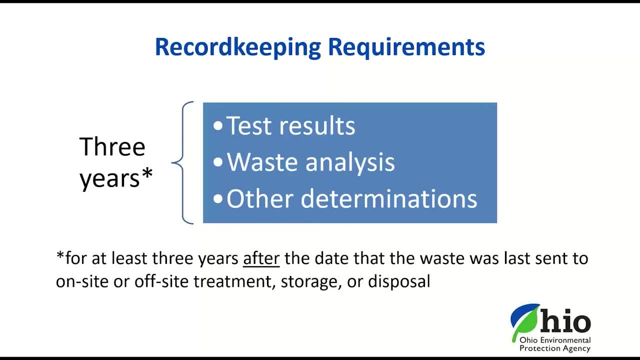 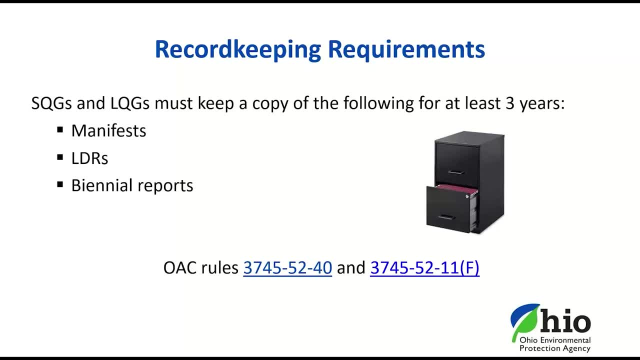 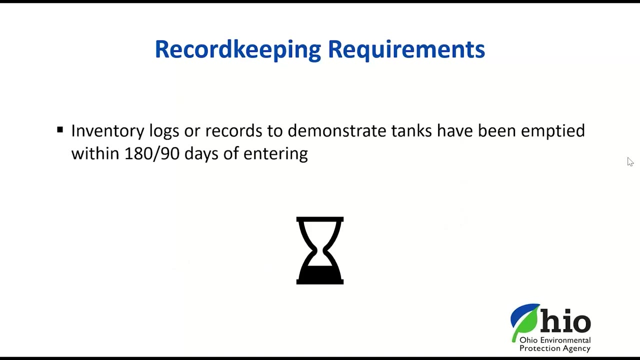 Slide 79, Slide 79, Slide 90, Slide 91, Slide 92, Slide 78, Slide 79, Slide 72, Slide 75, Slide 69, Slide 57, Slide 78, Slide 61, Slide 78, Slide 79, Slide 78. required timeframe. In addition, large quantity generators need. 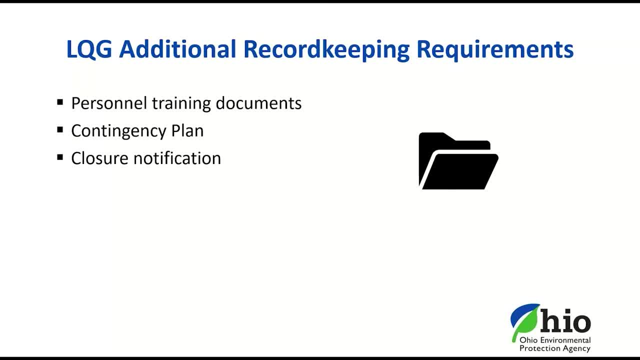 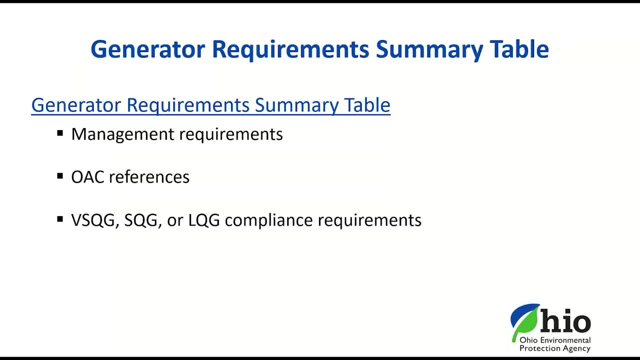 to maintain their employee training records, contingency plan and closure notifications. I've linked a requirement summary table to this slide. It's a helpful and comprehensive overview of the roles. It breaks down the various management requirements and lists whether very small quantity generators, small quantity generators or large quantity generators. 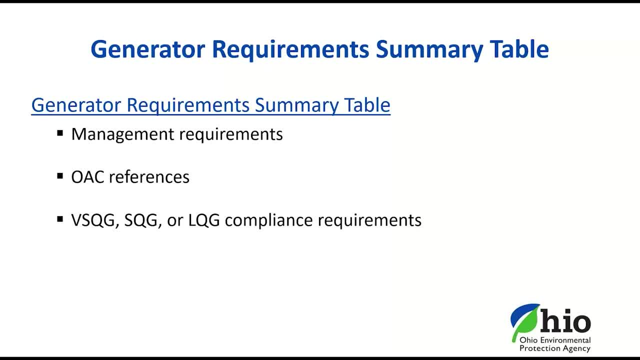 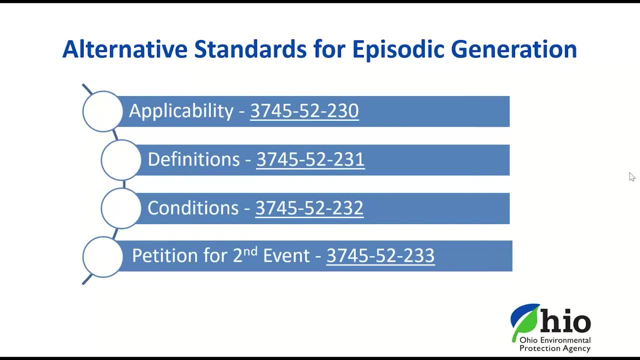 must comply with them And it also links back to the role citations. As part of the generator improvements role that were adopted in October 2020, episodic generation provisions were created to allow more flexibility for very small quantity generators and small quantity generators who have episodic events. 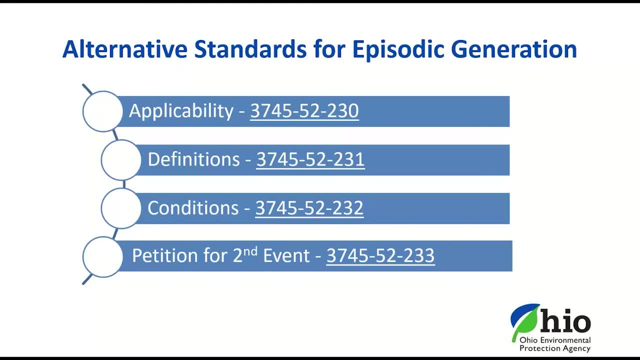 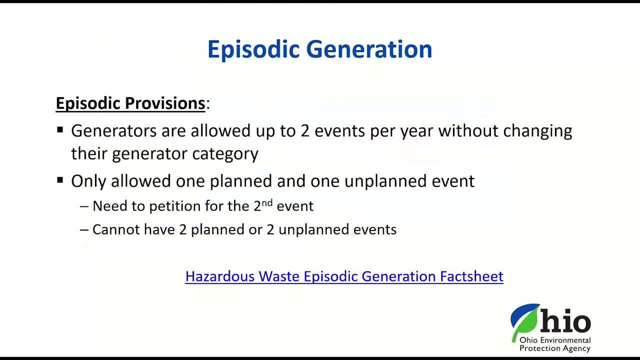 An episodic event is a scenario where an episode is generated and a generator is generated. An episodic event is an activity that does not normally occur that causes a generator to exceed the calendar month quantity limits for hazardous waste generation. Under these provisions, you are allowed two episodic events per year without changing. 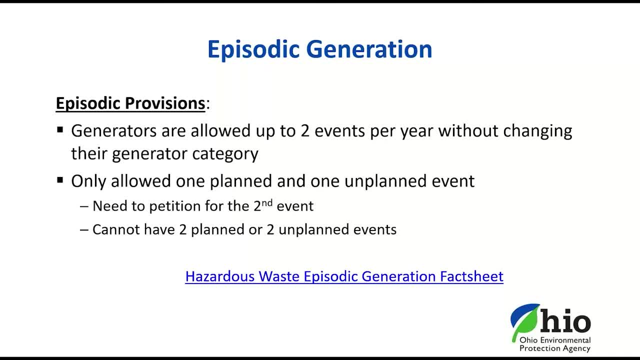 your generator category, but you can only have one planned and one unplanned event and you need to submit a petition for the second event. The linked fact sheet contains information on how episodic generators are generated and how episodic generators can be used. The link is in the description of this slide. 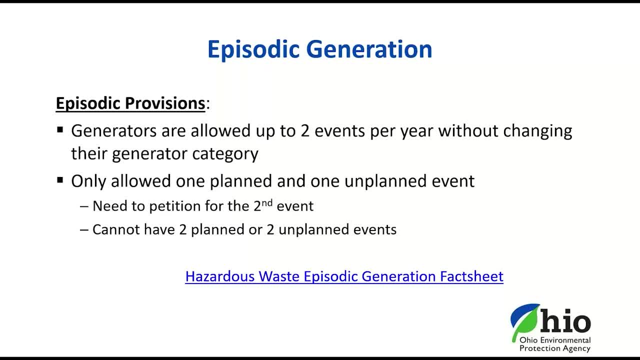 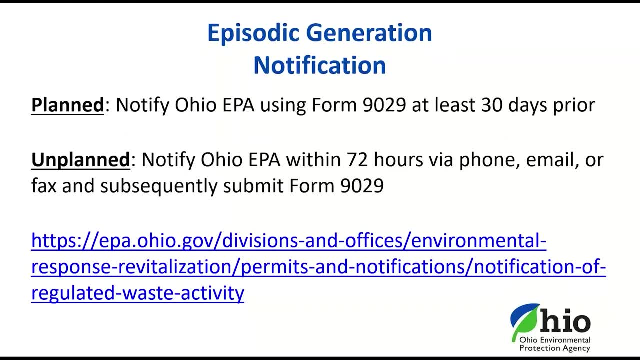 When you are preparing for an episodic event, you need to notify Ohio EPA at least 30 days prior to submitting Form 9029 and the episodic generator addendum. Both of those forms are located on the linked webpage. For an unplanned event, you need to notify Ohio EPA within 72. 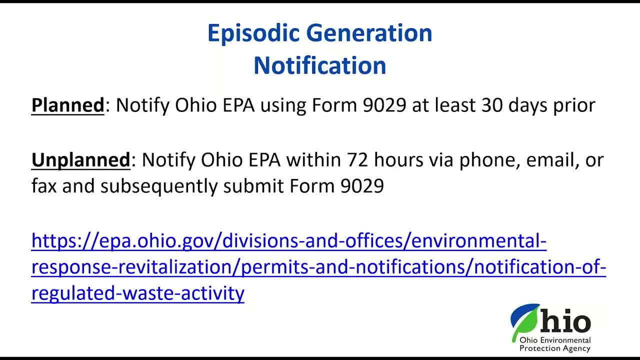 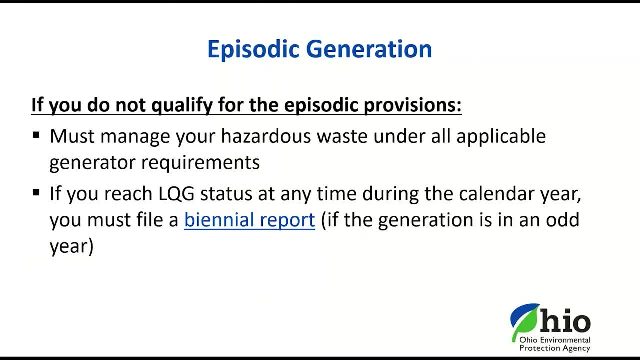 hours by phone, email or fax and follow it up with the required forms. If you don't qualify for the provisions, you need to manage your hazardous waste under the applicable generator requirements for whatever category you have bumped up into, And if you are a large quantity generator in an odd-numbered year, you would need to. 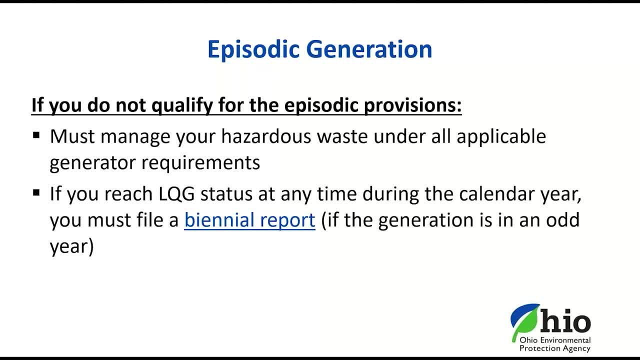 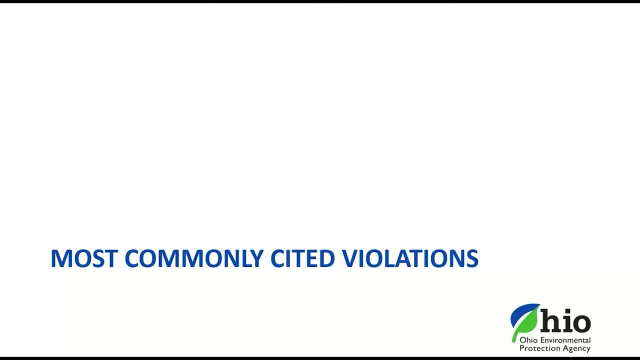 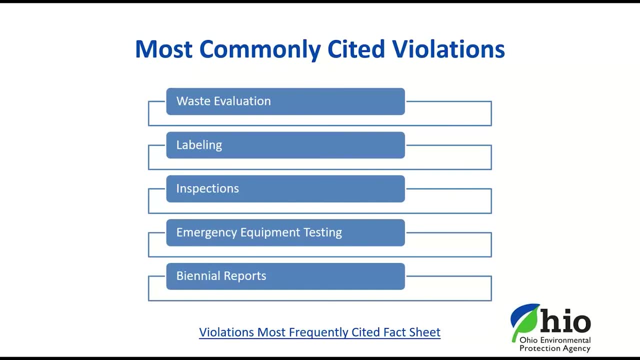 submit a biennial report in the following even numbers. Now I'm going to highlight the violations that Ohio inspectors cite the most. Throughout years of hazardous waste inspections, inspectors have identified the number one violation as failure to properly evaluate waste- over twice as much as any other violation. 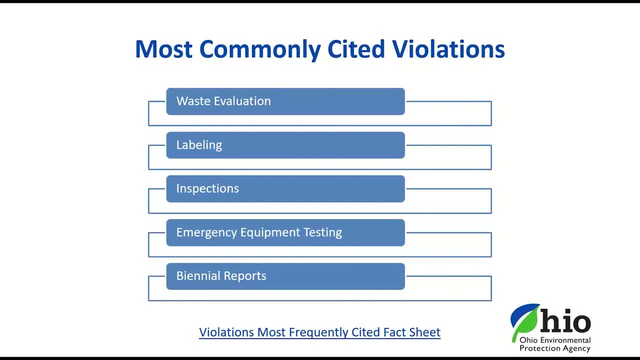 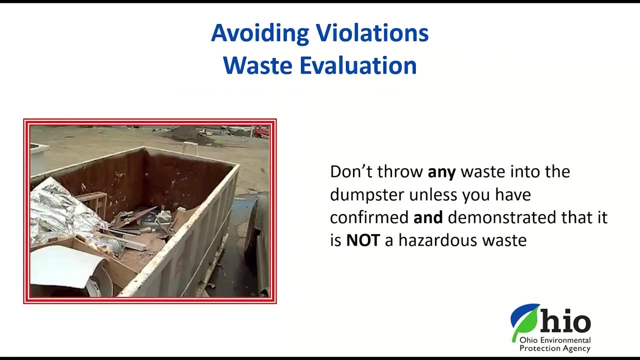 Other common violations include improper labeling and management of containers, not conducting weekly inspections, not testing or maintaining emergency equipment and not using the right equipment. Since it's the most common violation, I really do want to strive home that it's very important to not overlook waste streams. Don't put any waste into the trash before you confirm. 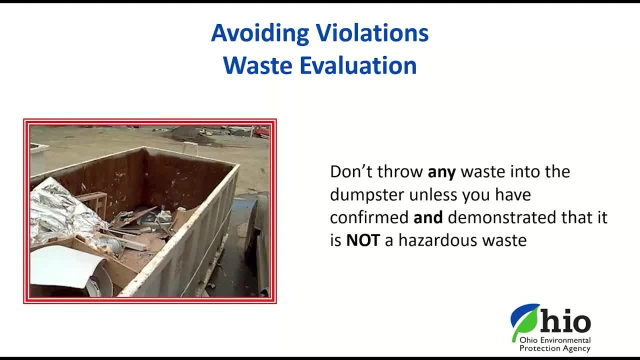 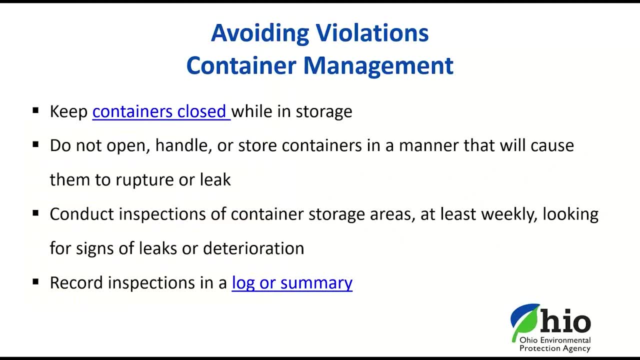 that it is not hazardous. This is something that should be communicated to all employees who could possibly dispose of wastes To avoid container management violations. the simplest thing you can do as a business is to file a biennial report. You can file a biennial report in the form of the following: 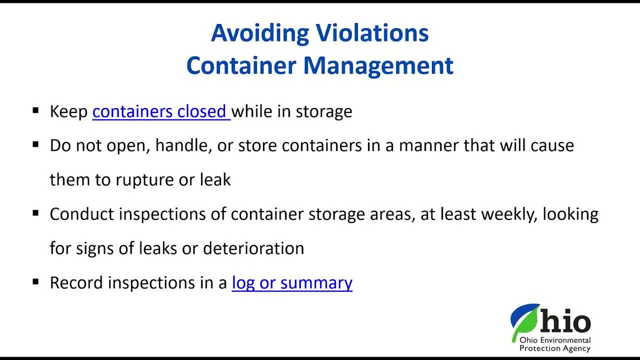 form. The first thing you can do as a business is to communicate to employees how hazardous waste containers should be managed, so that everyone is aware to keep containers closed and handle them in a manner to prevent damage or possible leaks, Because it only takes one person to make a mistake and leave the drum open. that could 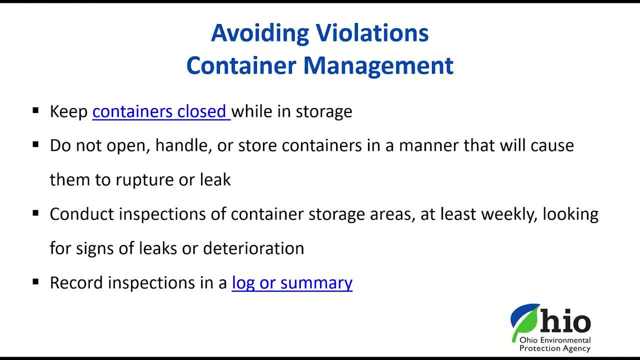 result in a cited violation. It's also a good idea to have a backup person, or maybe multiple backup people, to conduct the weekly inspections. Someone may be out sick or on vacation on the day that inspections normally take place, So having that system in place could prevent a gap in the inspection records. 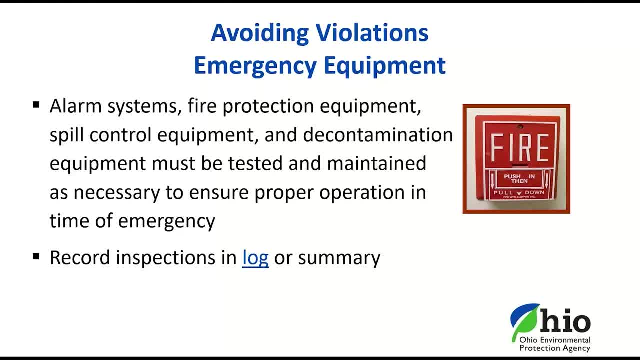 To avoid emergency equipment violations. you will want to make sure that you are inspecting your alarm systems, fire protection equipment, spill kits and decontamination equipment at the appropriate intervals and also documenting those inspections. Something you could consider for your spill kits is to use tamper seal tape so you can easily tell if someone has. 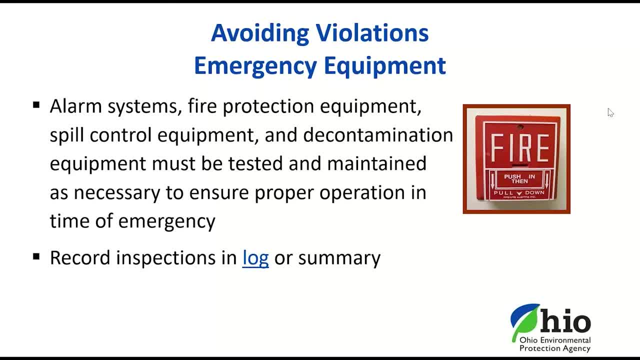 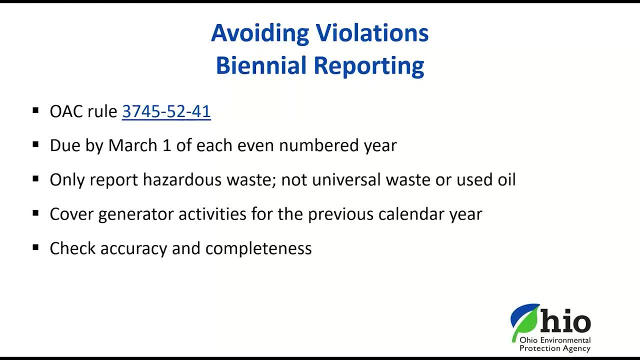 opened the kit insignia of the equipment if it is not available in the system, If it is not available at the. To avoid biennial report violations identified during an inspection, you will want to make sure you submit the reports by the March 1st deadline and even-numbered years. 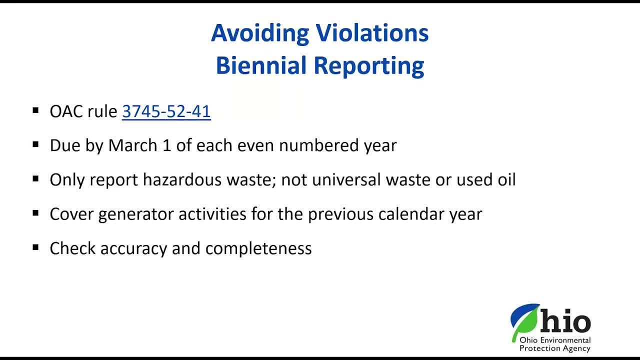 Once again, if you have not yet submitted a report, please do so To make sure that your report is accurate. keep in mind that you should only include your hazardous waste streams, so no universal waste or used oil should be on it and you. 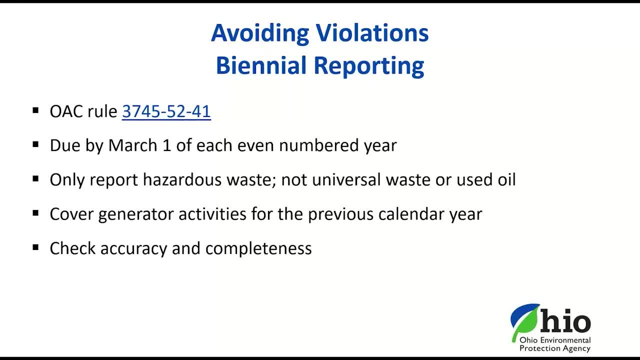 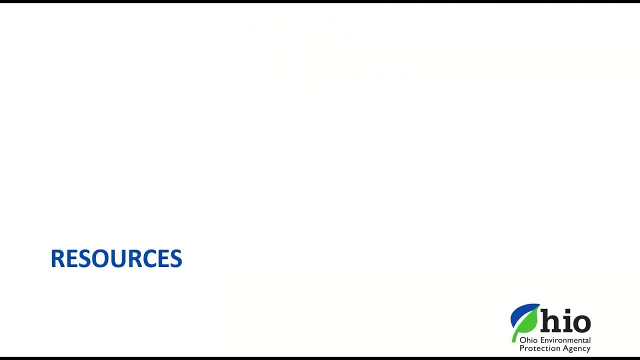 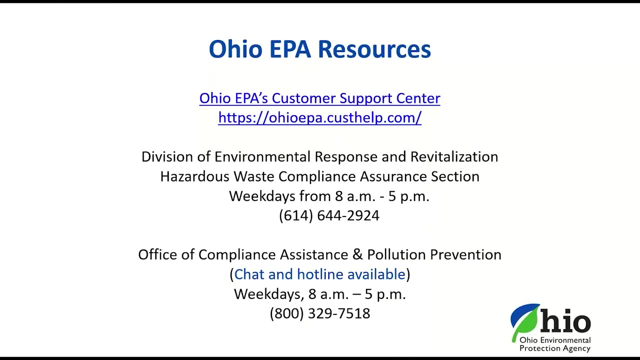 should always double-check it for accuracy before submitting. The next few slides have some links to useful resources I felt might be helpful, so we'll have them in the downloadable content and you can check out those webpages. If you do have questions, please reach out to us. 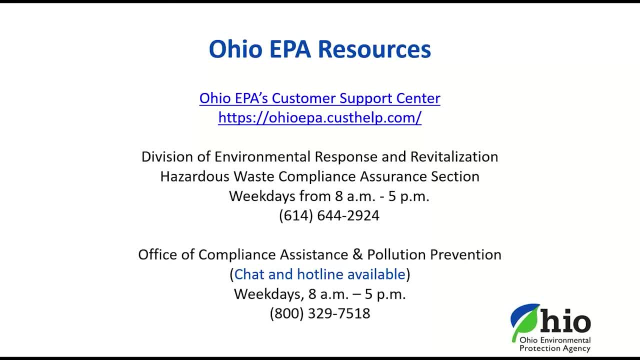 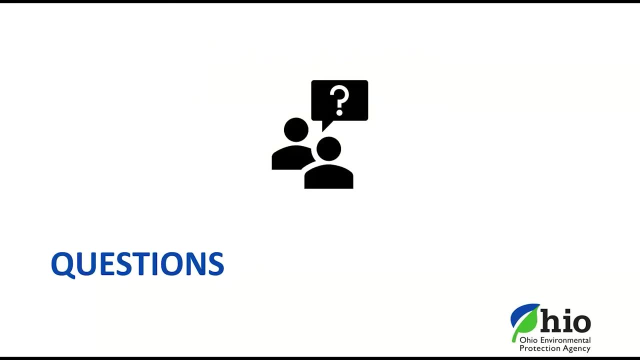 You can search our knowledge articles, You can submit questions there or you can reach out to speak with my section directly during the week or during this presentation right now, and you can also take advantage of OCAP's Confidential Compliance Assistance, Hotline and chat service. 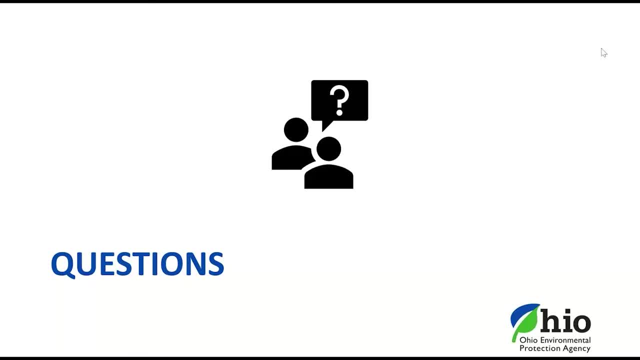 Okay, Thank you so much, Bill, for your great presentation, and thank you, Tammy and Christy, for helping address submitted questions. We have a lot of questions coming in. We unfortunately don't have time for more questions. We'd also like to bring to your attention our Encouraging Environmental Excellence Award. 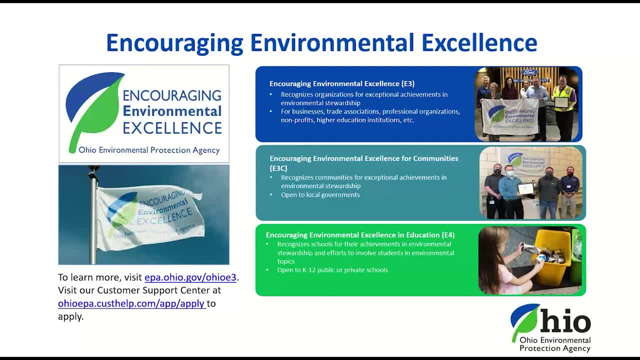 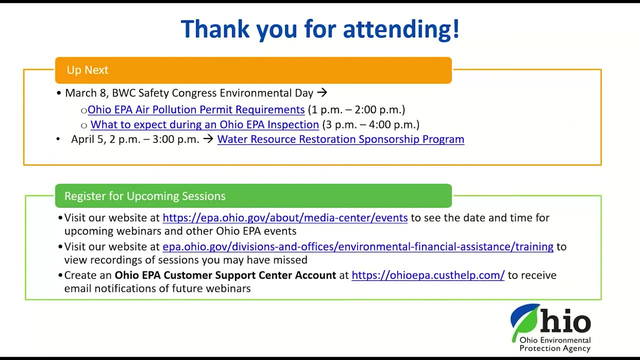 program which recognizes entities for exceptional achievements in environmental stewardship. Please go to our website at the link on the slide to learn more about this program, and please join us for some more webinar sessions today as part of VWC's Ohio Safety Congress. 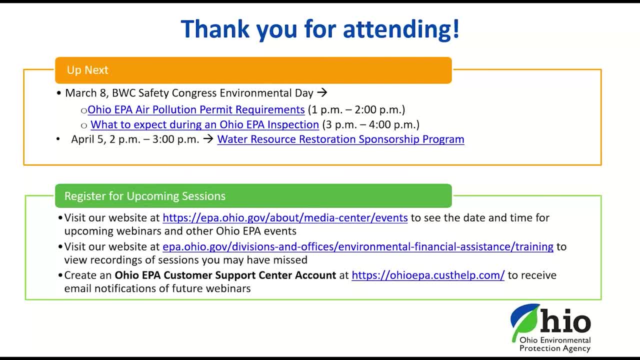 We have an air pollution program. We have a lot of questions. We have an air pollution permit requirement session from 1 to 2, and what to expect during an EPA inspection, from 3 to 4.. And then on April 5th, we have a webinar on our Water Resource Restoration Sponsorship.